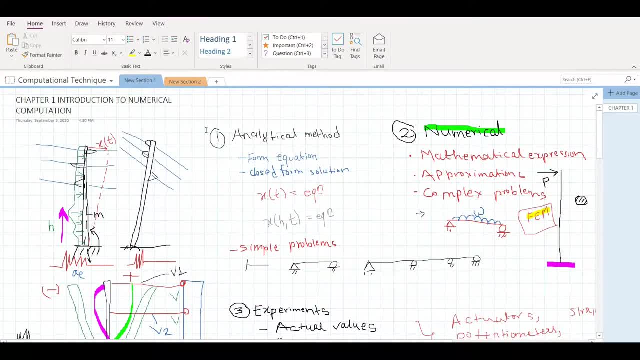 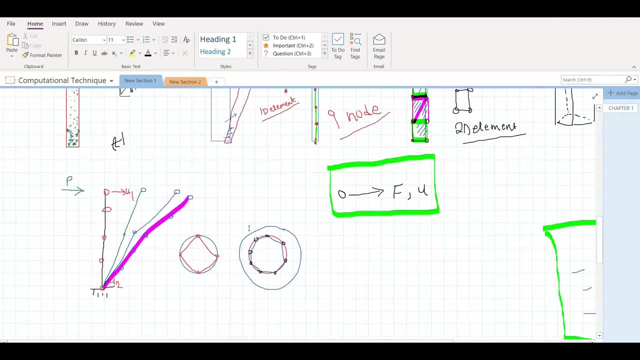 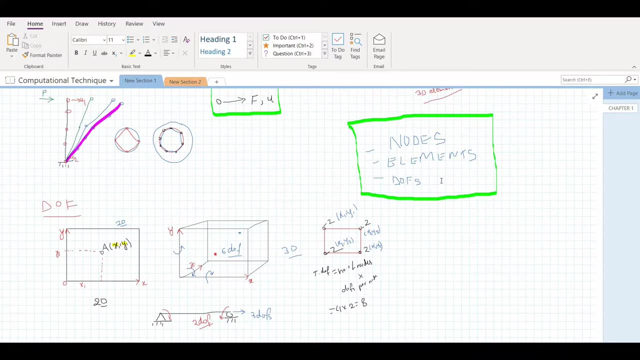 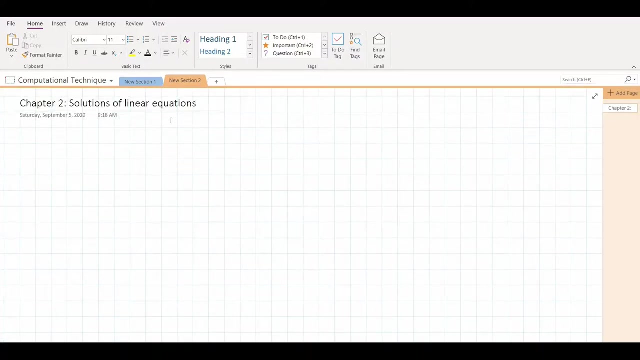 Hello everyone. In the last session we briefly discussed about finite element method and we learned about certain terms which are very essential in finite element method, which are nodes, elements and degrees of freedom. Now, today, we move into second chapter, which is on solutions of linear equations. What are linear equations? As you might already know that the equations such as this one, which varies linearly, with a certain slope and certain initial value, are known as linear equations. 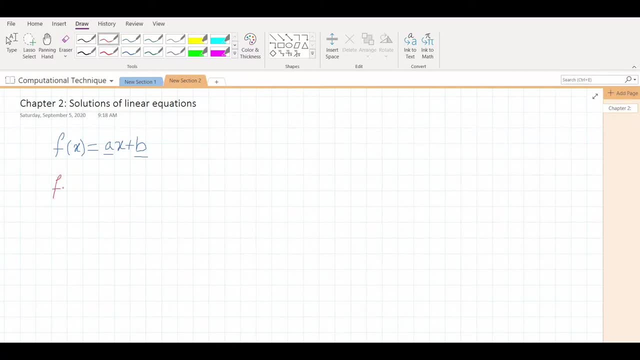 Now the linear equations may depend upon many variables, which may be x1,, x2, x3 to xn, where you can have a1, x1, a2, x2,, a3, x3 to xn. Now the linear equations may depend upon many variables, which may be x1, x2, x3 to xn, where you can have a1, x2, x3 to xn, where you can have a2, x2, x3 to xn, where you can have a2, x2, x3 to xn, where you can have a2, x2, x3 to xn. 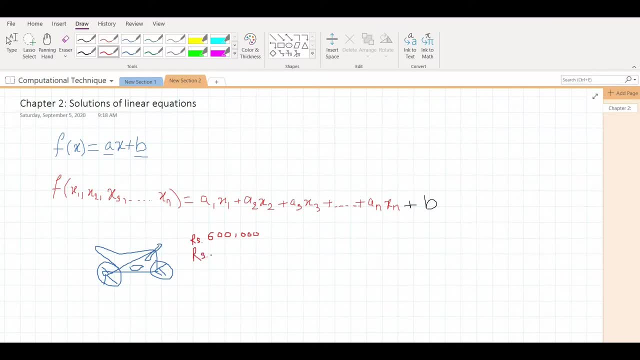 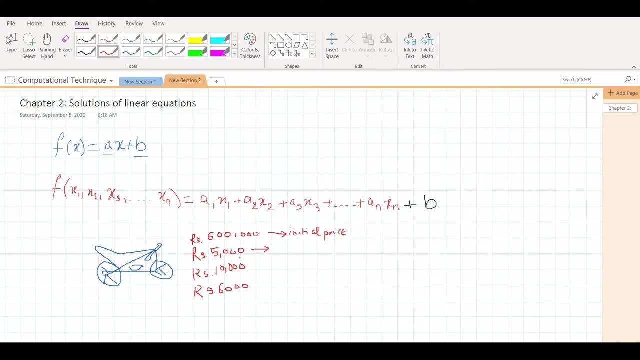 That's your insurance and this is your fuel. We convert this to per month, so it will be RS1000.. If you want to find out how much will be the total cost for your motorbike if you have it for two years, let's say two years- 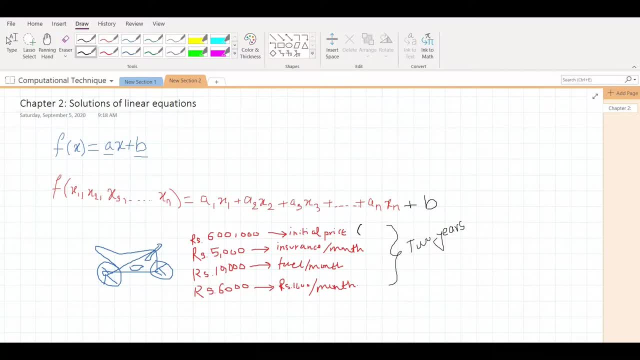 Now, if you look into the variables now, this will be a constant that you paid initially, which will be the y intercept, and then these terms will have a single variable, t, which is time in months. So you can form equation like: total cost will be equals to. you can add these up and this function. 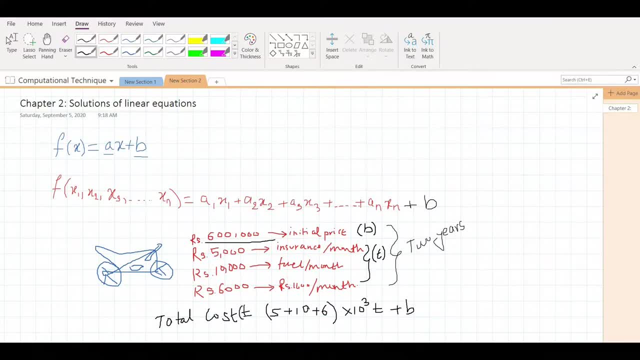 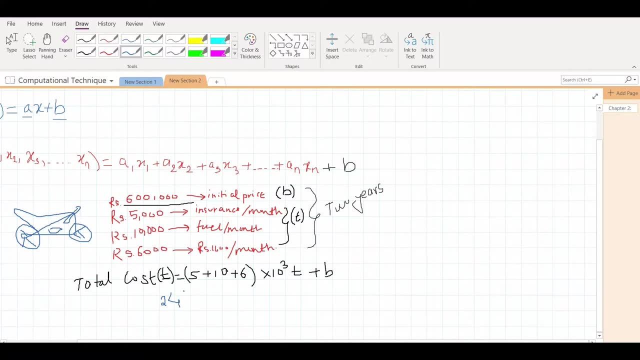 depends upon time. Now here you can plug in two years, that will be 24 months. This will be your total cost of owning a motorcycle for two years. Now you can have other variables as well. Let's say what you do is you rent your motorcycle? 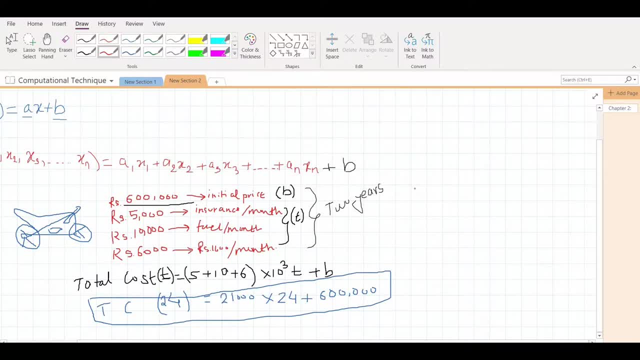 to total or uber and you charge them per kilometer of distance that he has traveled. So let's say initially, if the mileage was 90,000 kilometers and you charge him at a rate of RS 50 per kilometer, So this will be your earning. 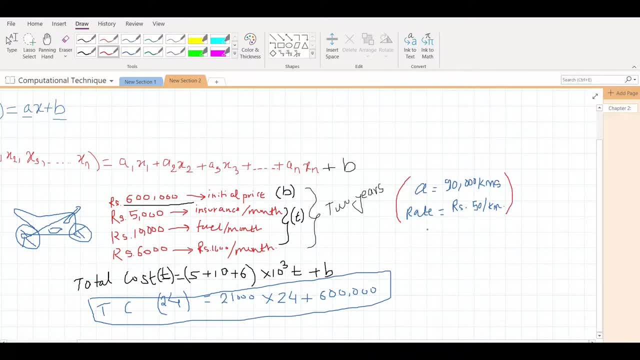 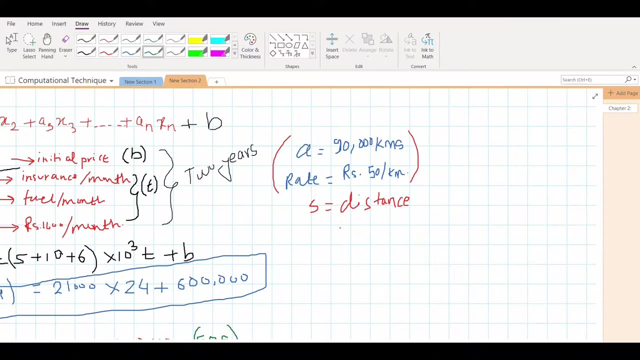 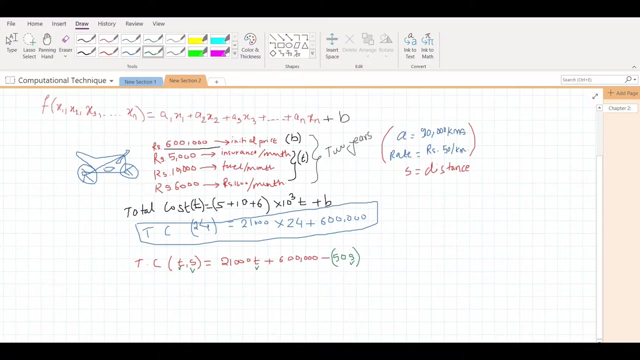 here, and then if we include this distance s as distance as a variable, then your equation will be modified into where s is the distance the guy who has rented your vehicle has traveled. so in here we have two variables, T and S. therefore linear equations will have a generic form of something like this. so 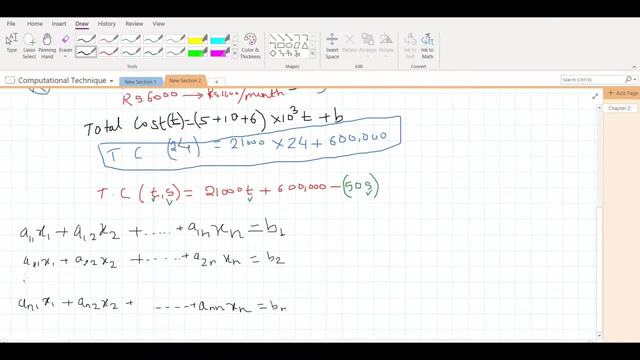 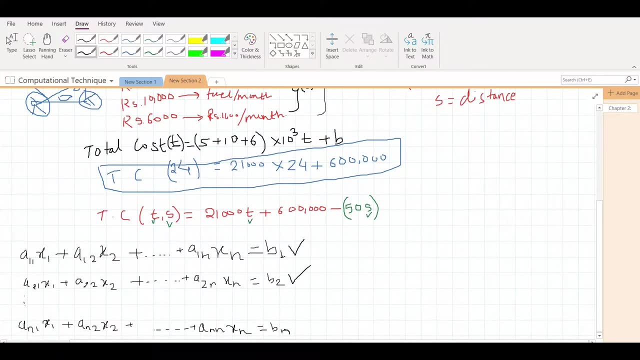 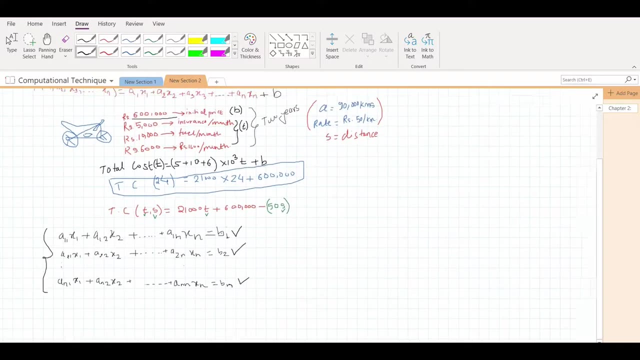 you can have a lot of combinations. for example, if you have n number of vehicles that you rent or that you have bought, so this can be for your motorcycle, this can be for your car, this can be for your truck, and so on. so they can be many equations like this, and then you may have to solve them in FEM. we. 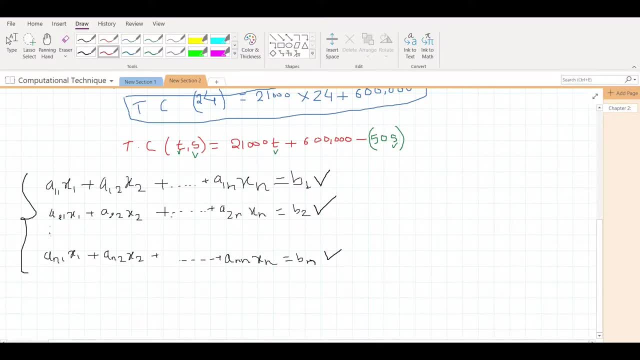 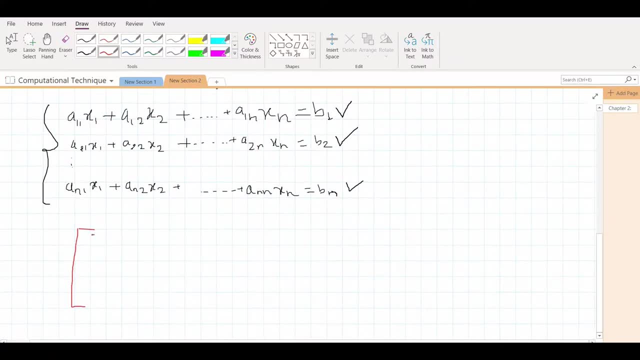 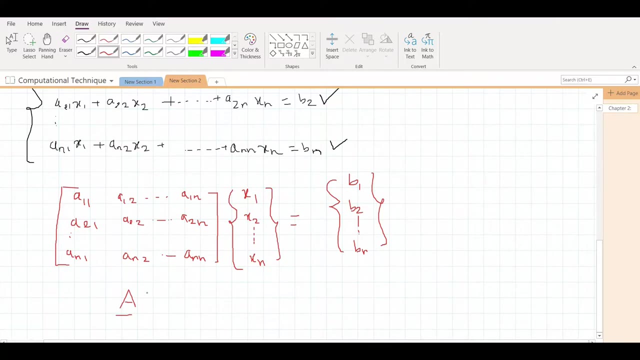 generally write these equations in matrix form. we try to solve them in in matrix form. so matrix is the basic here. so when you write this in matrix form you'll get is: this equation can be represented in matrix form like this: so there's a matrix: X vector equals to B vector, where you have to solve for X factor. here you: 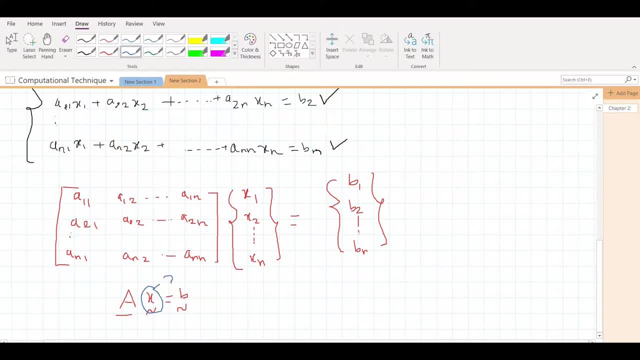 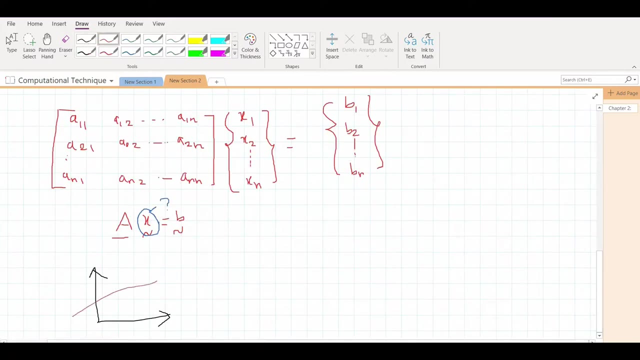 have to find this now. there can be many solutions to it. there can be one single solution. for example, if you have two linear equations which, when you plot in your XY graph, they mean something like this first equation maybe like this second equation may be like this, so they will only have one solution like this. so 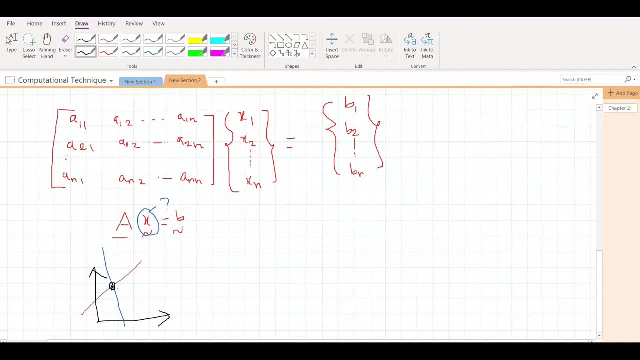 these are known as equations having unique solutions. so this is unique: they only have one solution, and for other cases, like when you have two equations which are parallel to each other, then they will never intersect, which means there will be no solution, and then you can have two equations like this, which 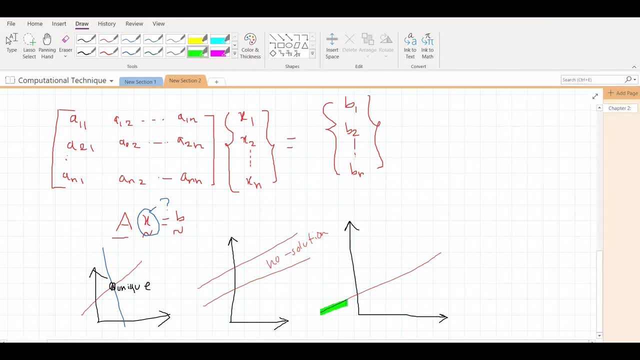 overlap each other. so that's the first one, and then you also have the second one going on top of it, which means every point in the black line will be coincident with the point in the green line, so they will have infinite solution. the way to solve. 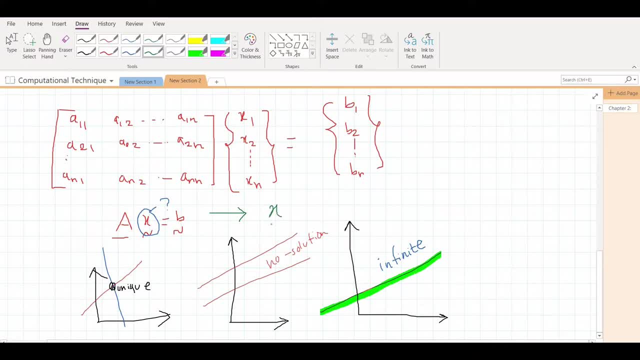 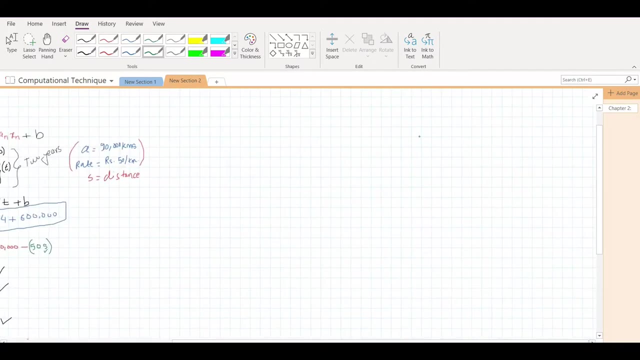 this is X vector will be equal to. if you take this matrix on the right side, it will be A inverse B vector. that's how you solve it. now there are many solution techniques to solve them. the first technique we're going to learn is the Gaussian elimination method. in this method, what we do 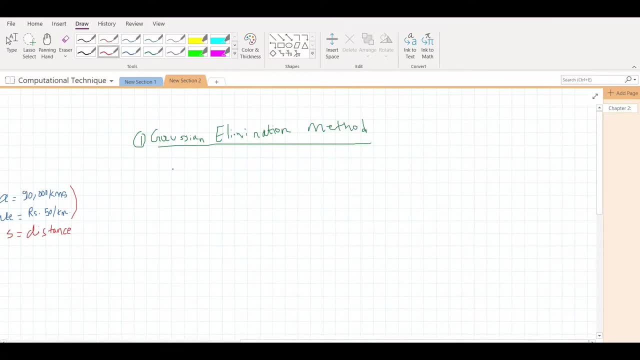 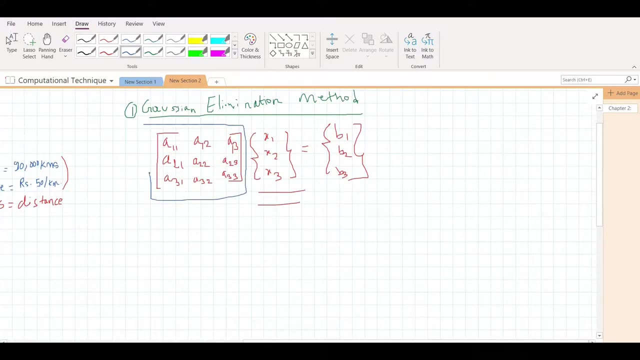 is, if we have a equation like this and you want to solve for your X values, then what we have to do is we have to use some mathematical properties of matrices and convert this matrix here into this form. so when you apply different mathematical properties of rows and columns, you'll end up with 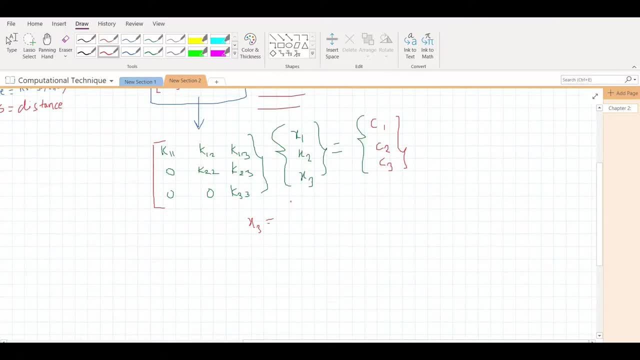 something like this. so you can easily solve for X3 first and we can see that the X3 is equal to X3 by K33. and once you know X3, we can open the second row now for this one, since you know the value of X3 from this. 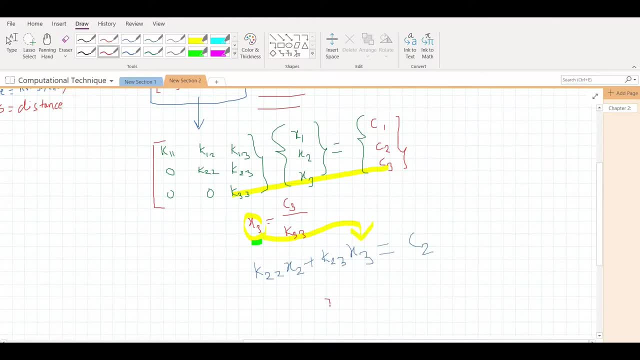 equation here. you can substitute it here to obtain your X2. so X2 will be equal to. similarly, once you know X2, you can solve for your X1. so your X1 will be something like: now you have solved your problem. here you can get your x1, x2 and x3. so this is one of the methods. 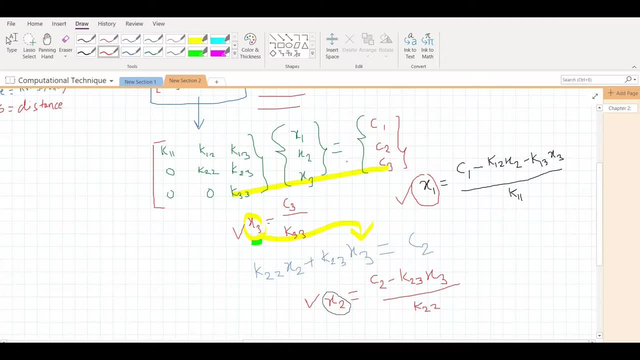 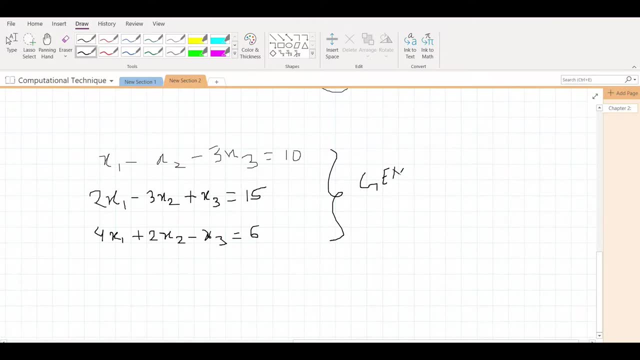 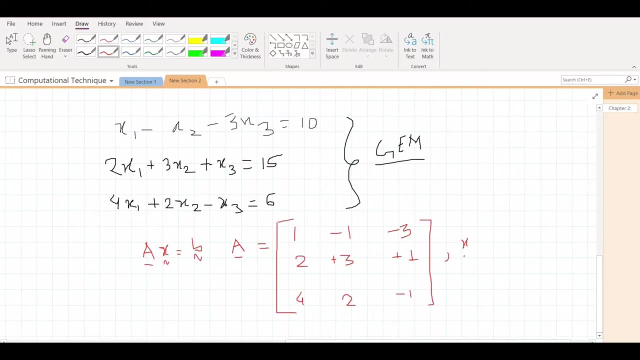 let's look at an example of this one. let's say we have this equation and we have to solve it using gaussian elimination method. so the first step is to form your matrix equation like a matrix will be equal to x, vector will be equal to v vector will be equal to. we actually don't have to write. 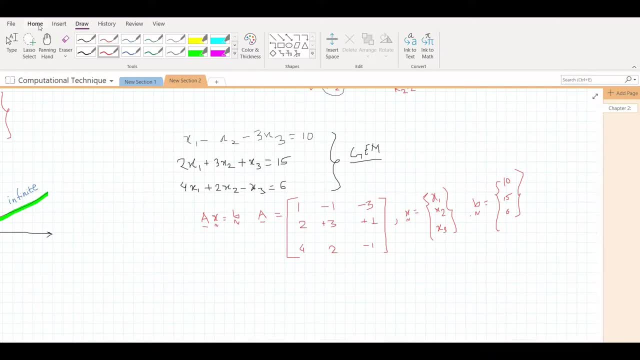 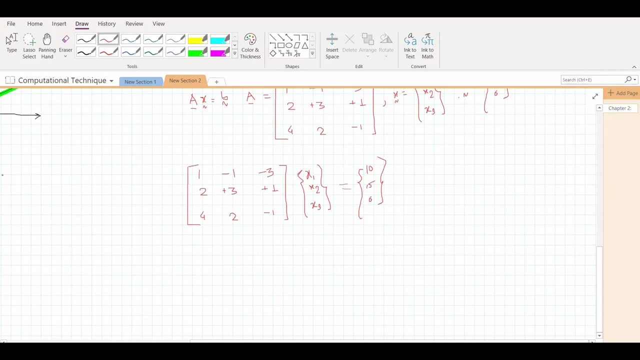 it this way, you can directly write your equation like now. let's try to solve this now. the first step is to make this one zero. to do this, we have to either add or subtract these values, rows. let's say this is first row, second row, third row. so to get this, we have to perform. 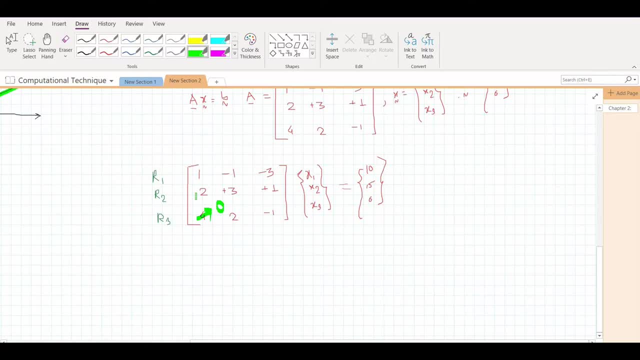 some mathematical formulations. we can do two operations. we can either do some manipulation in r3 or r2, keeping r1 same, or we can do manipulation of r1 and r2, keeping r3 same. so first we're going to try to make this one zero. what we can do is that. 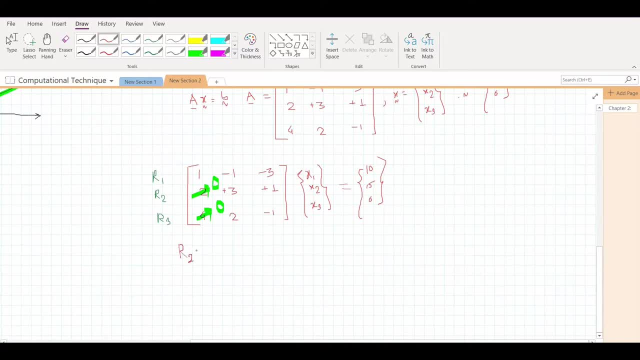 if we look in r2, so our new r2 can be r2 minus 2r1. so when you subtract twice of this row from this row, then it will be 2 minus 2, then you will get zero here, and similarly your new r3 can be r3 minus 4r1. so here we have kept r1 the same. then what you'll have. 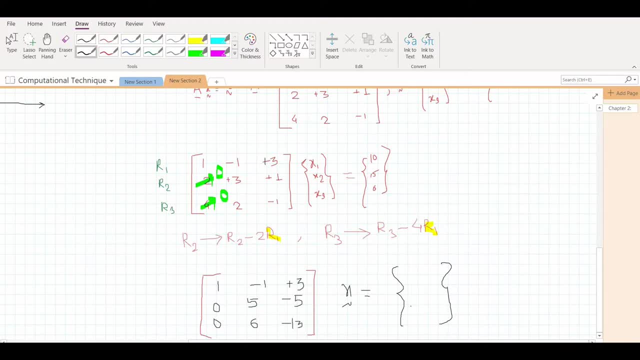 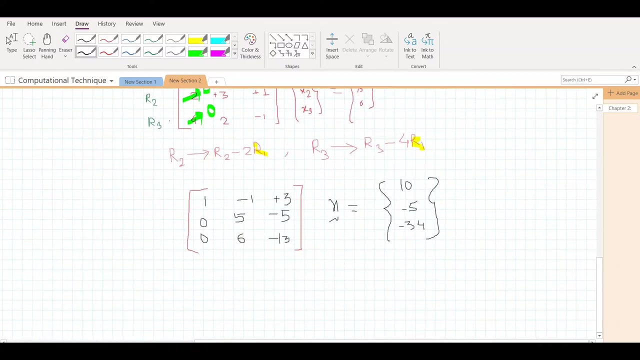 here is. here also, you have to do the same. so here you get 10, here you get 15. minus twice of this, you get minus 5. and then here 6 minus 4 times of this 40. so that is minus 34 again. let's make this one zero. now, to make this one zero, we have to subtract this one, because 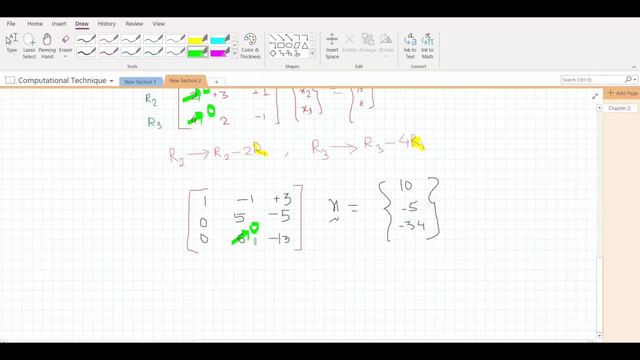 we want to retain our zero here, so we have to do manipulation in r2. so what we'll do is your new r3 equal to r3 minus. let's say we have to multiply this by 6, by 5 r2. therefore our new matrix. 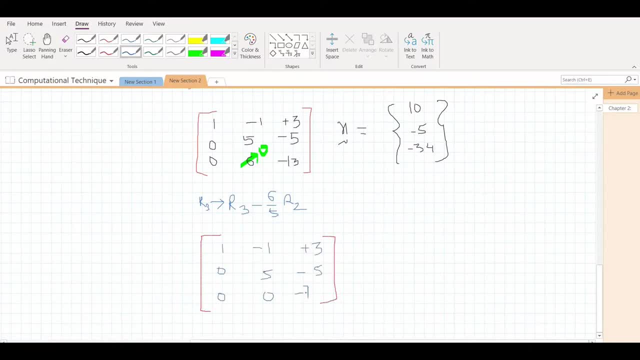 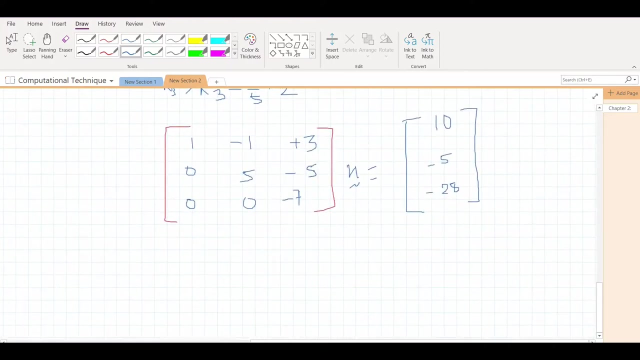 will be x vector equal to 10 minus 5, and here you'll have minus 34 minus minus 6, that will be minus 28. now you have your equation. now you want to solve it? so here we can write minus 7. so this is: 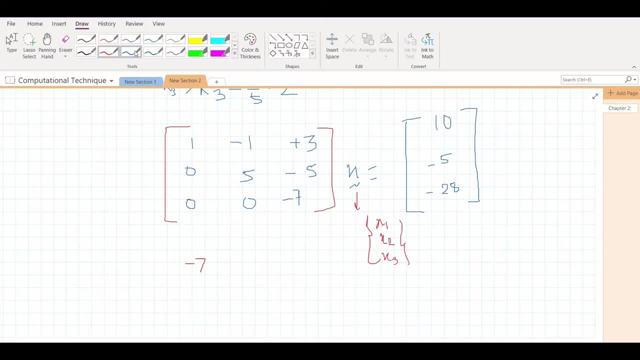 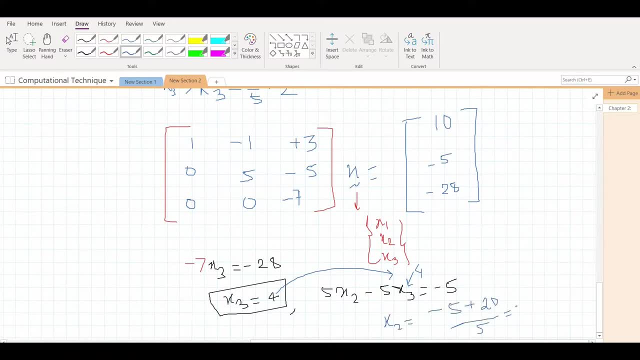 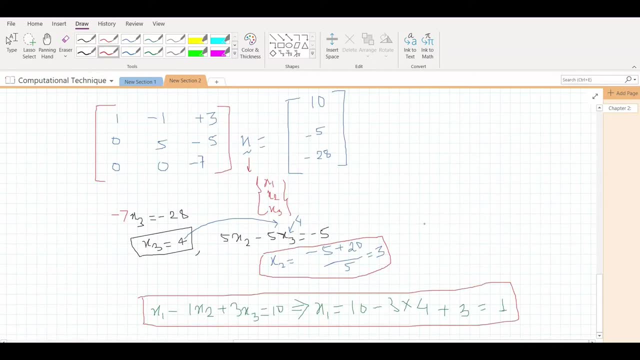 and then you'll get your x2. that will be equals to 3, and again x1 will be equals to 1. therefore, your x vector will be equal to 1, 3 and 4. so that's your solution. now there is another method, which is known as gauss jordan method. 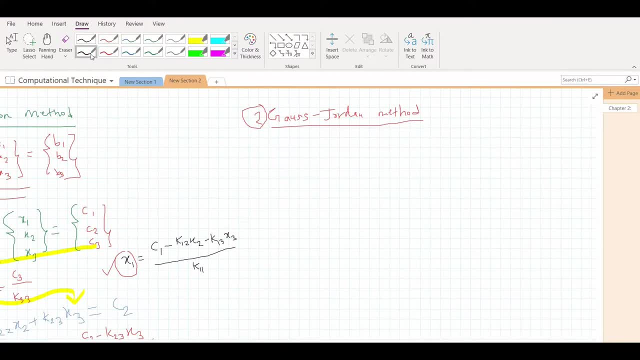 this method is similar to gaul's elimination method, but here your final a matrix will be of this form: x1, x2, x3 equal to c1, c2, c3. so here you can directly solve the equations. so x3 will be equal to c3 by k3. 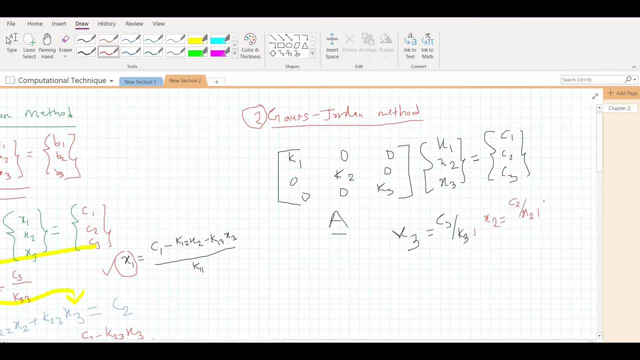 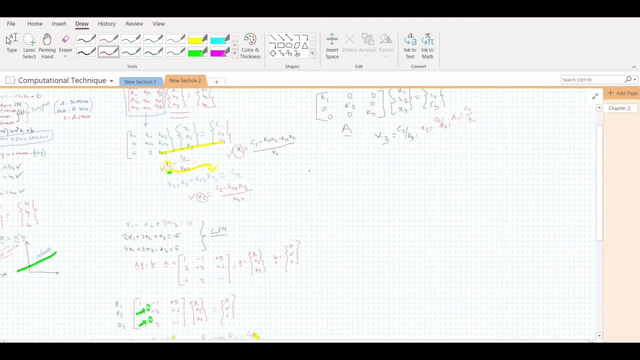 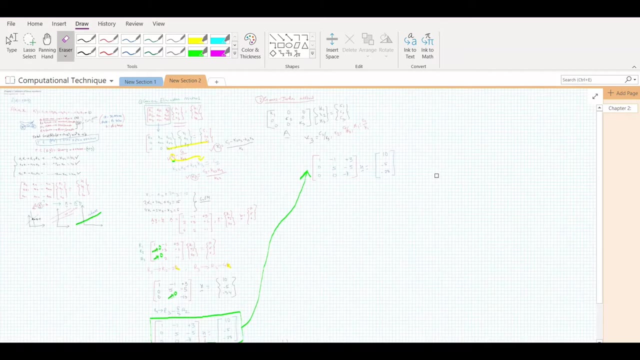 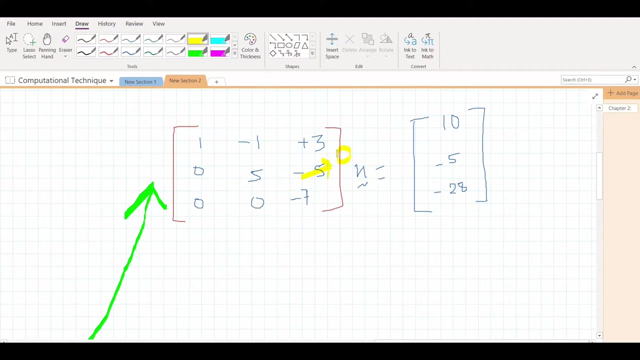 x2 will be equal to and your x1 will be equals to c1 by k1. you can try solving the same problem and finally obtain this kind of matrix here. so let's try it, so you can start from here. so our target now is to make this one zero. now, to make this one zero, what you can do is 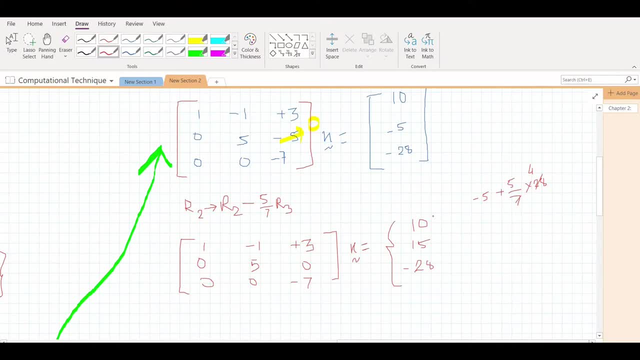 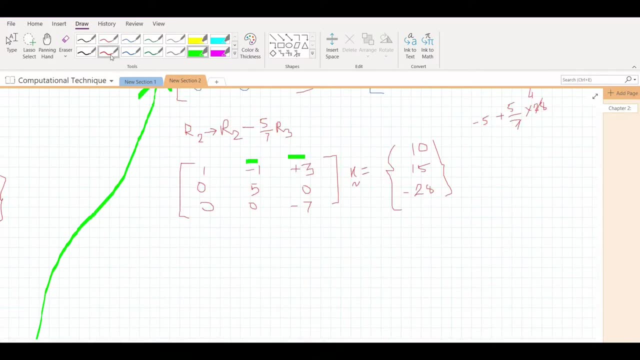 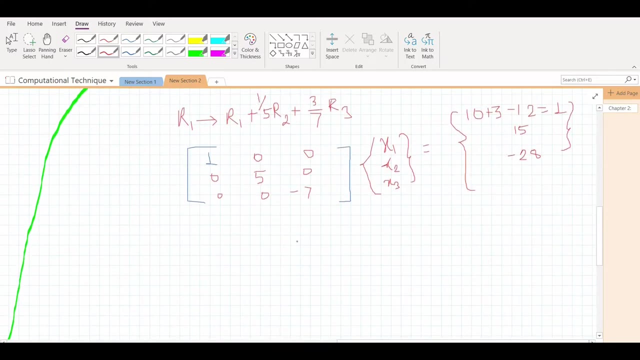 so after this, what we'll get is: now we have to make this one and this one zero. to do this, what you do here is: now you can solve this easily. so you'll get x3 equals to 4, x2 equals to 3 and x1 equals to 1, which is the solution that we obtained earlier. 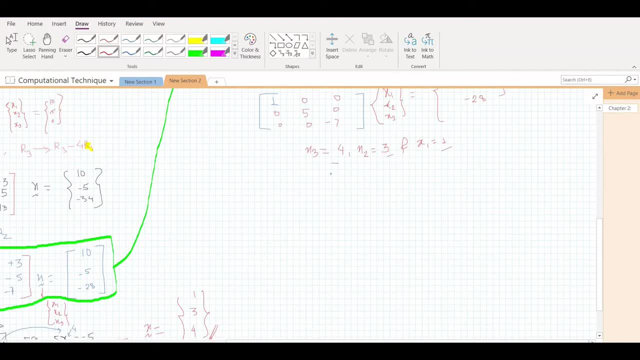 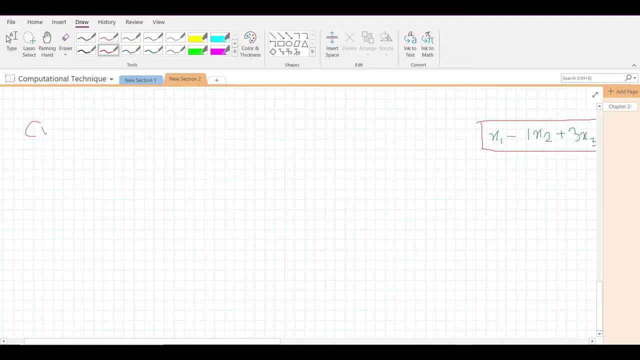 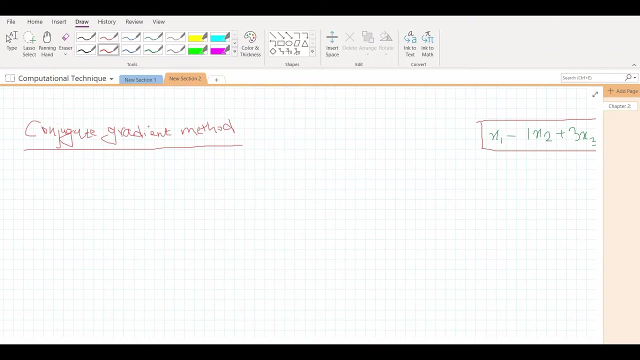 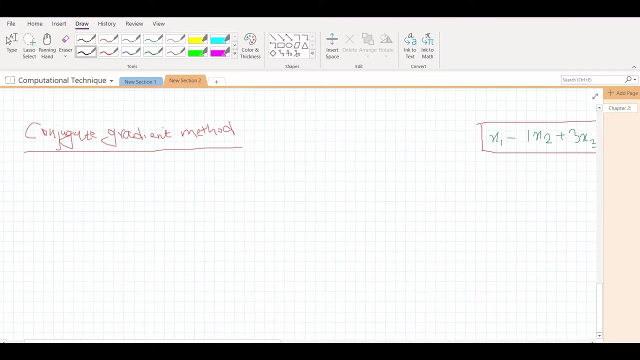 we have one, three, four, one, three, four now. this is known as gauss jordan method. now we'll move into conjugate gradient method. conjugate gradient method is one of the numerical methods to solve linear equations iteratively. gradient means slope, so these methods use slope to solve. 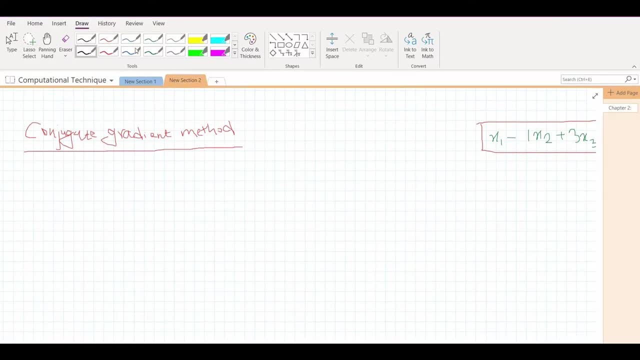 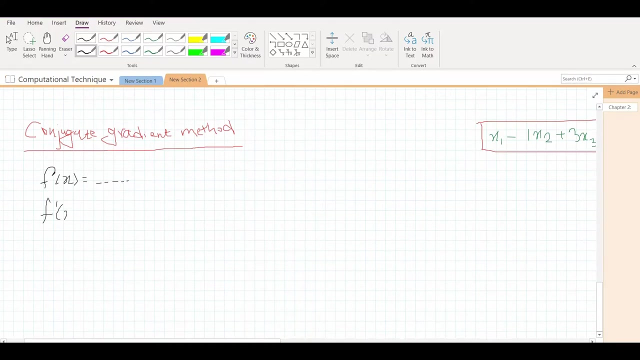 the problems generally, what to do is if you have equation like this, let's say fx, it goes to some equation then to find the minimum or the maximum value of fx, what to do is find the derivative and equate that to 0. we'll check this condition and 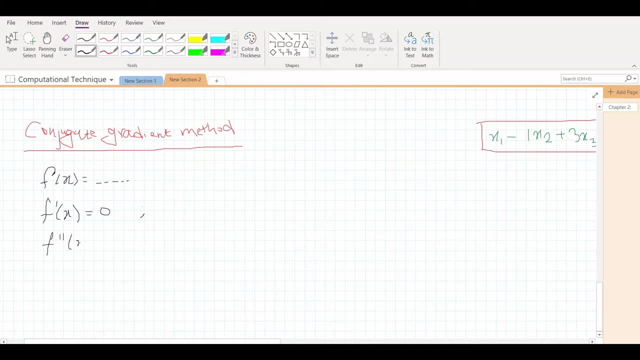 we also check its second derivative and see if it's greater than 0 or less than zero. if these conditions satisfy, then we find minimum or maximum. let's say your fx is this, and when you do a derivative and reach here, then the slope of this line will be parallel to x-axis. this will give you the 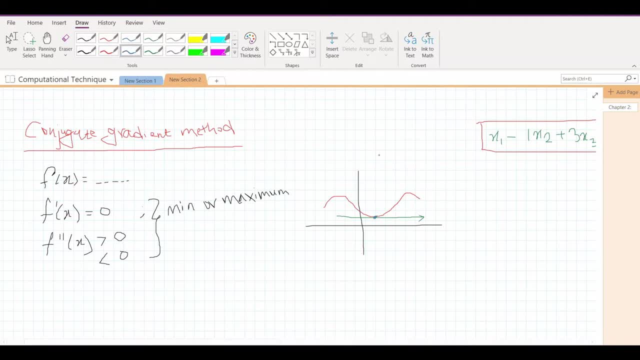 minimum value and in this range it will be also parallel to x-axis, and this will give you your maximum value. now, for conditions like like this, where there are no constraints, for example, your problem might say that you have to solve it such that x lies between a and b. if this be a, 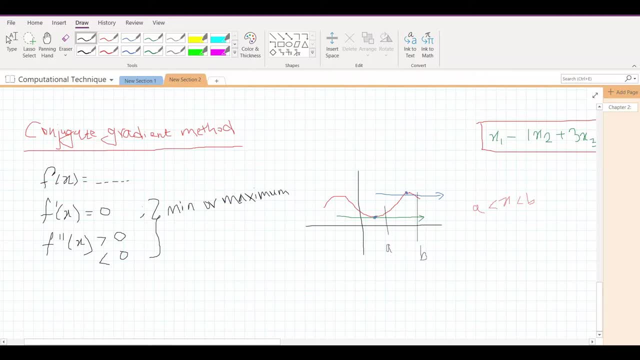 and this pb, then you have found your solution. and in such cases where these are not given, then your x can vary from minus infinity to infinity. now these kinds of problems are known as unconstrained problems, because your solution can lie anywhere here now these gradient methods make use of 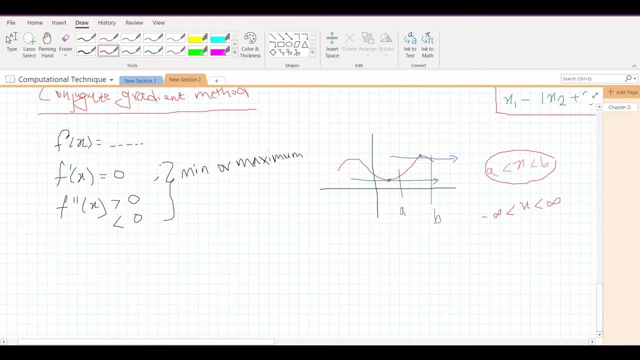 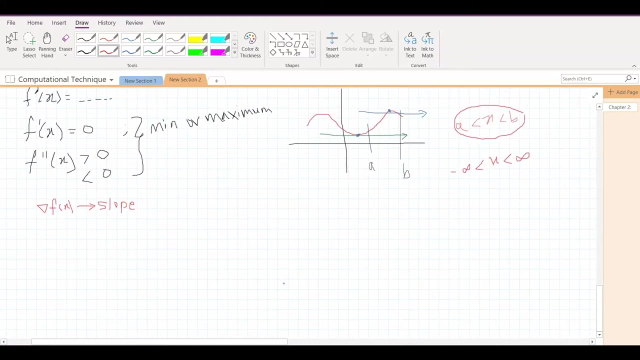 these derivatives to minimize or maximize certain equations. the gradient of fx is generally denoted by gradient mean slope. now we have a function, fx, and we want to solve it using the slopes or the gradients. let's say that your solution is in this space. now, if we try to calculate the function of thisfs, we need thezenia, and dy can be portioned. 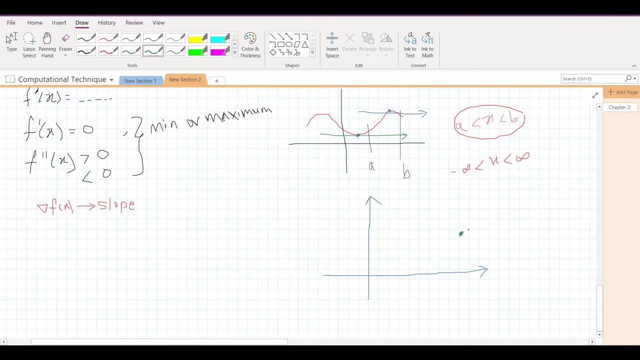 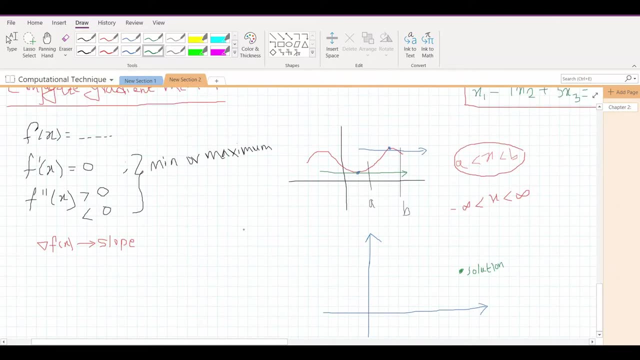 ordered by determinant n, and then sum them together and we have a function fx here. and then sum them together and we have a function fx here and in thatision grasses. so ourентrelative method. again, we are not going to implement this method. as we know, we can do it by taking an initial coefficient of x. 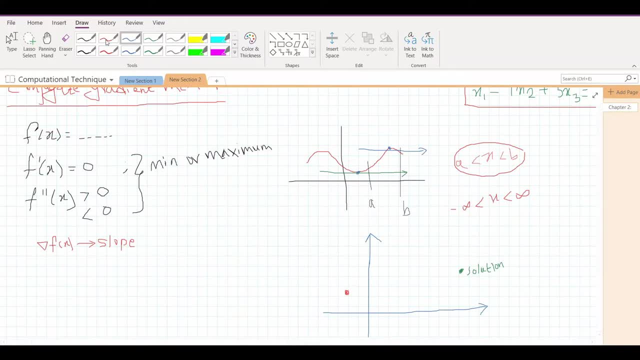 we're going to do this here. within this equation, we have to reach here now. to reach here directly, we have to know the path, but we don't know. that's why what to do is: first we find derivative of the function at this point here and move into this direction like this, and go to a certain point here and then 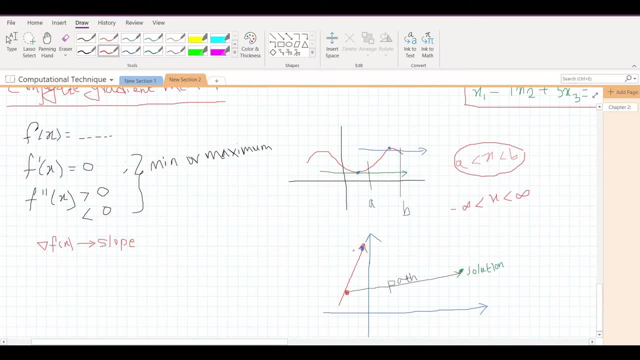 we'll find another slope and then maybe move into this direction and to a point here, and then we find slope of this point and then, moving this direction here, and then find slope here, moving this direction here, and then finally we may move in this direction and reach to our solution. 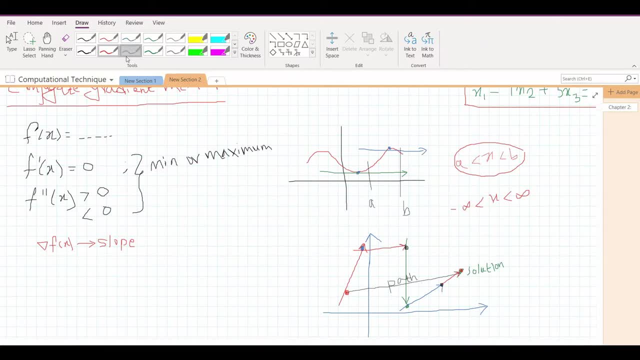 since we don't know this path, we have to start at a point x1 and then move to x2, then x3, then x4, x5 and then reach our solution, x2. so it took us one, two, three, four, five, five steps or five iterations to reach to our exact solution. 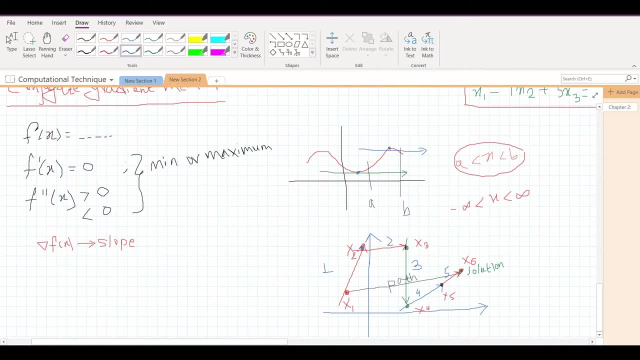 this is how the gradient method works. so if the slope of this line here is m1 and this length here is alpha one, then your x2 will be equal to x1 plus alpha one, m1. we know x1, which we can assume. we can assume x1 to be a certain value, like, say, zero. 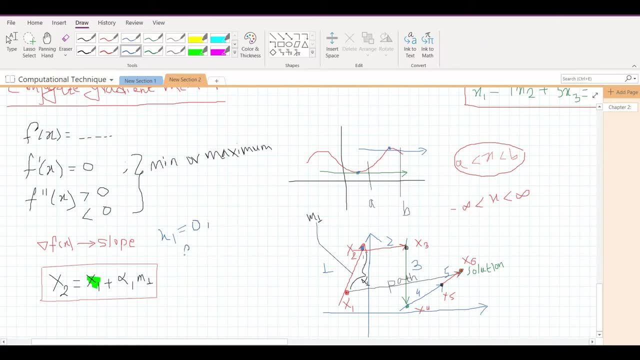 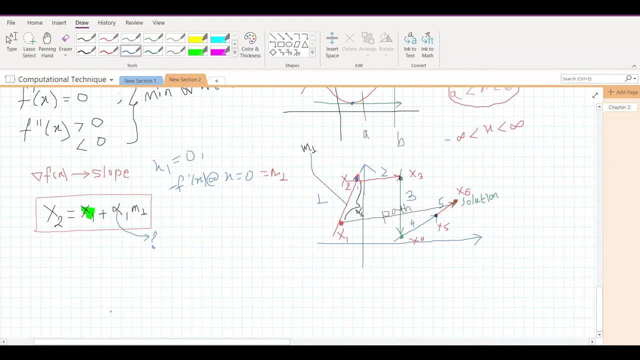 and we will know m1, which will be derivative of our function at x equals to zero, generally negative, which will be equals to m1. but we don't know alpha one, so we have to find alpha one. alpha one is kind of like your step size. we want to know how far we want to move in this direction so we can reach here faster. so in 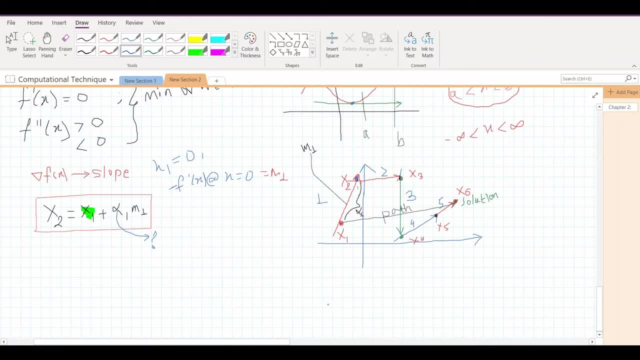 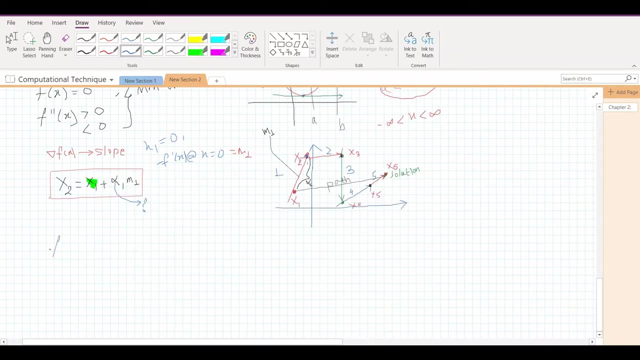 numerical methods to find alpha one. you can use Newton-Raphson method or bisection method and so on. and there are also analytical methods, and here we will directly use analytical method to find the value of alpha one. if i write f x2 equals to: 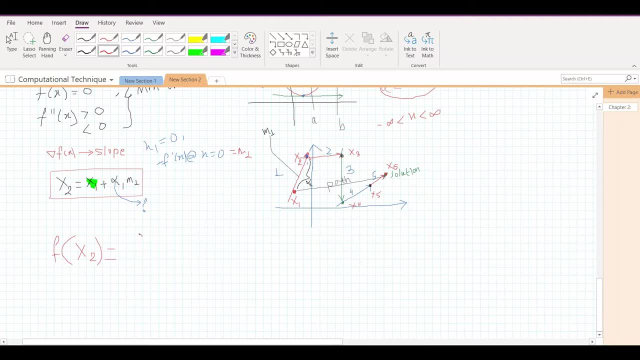 theю fn of x1 plus alpha one m1, then i can use taylor series to open this. i believe you have studied taylor series in your previous years. this will generally be matrix form. what to do is we can write here: f of x1 plus gradient of x1, alpha 1 m1. 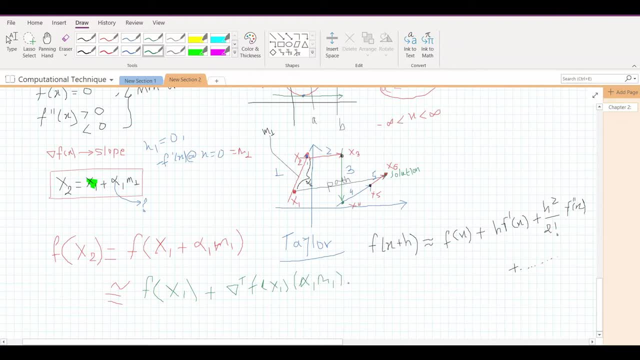 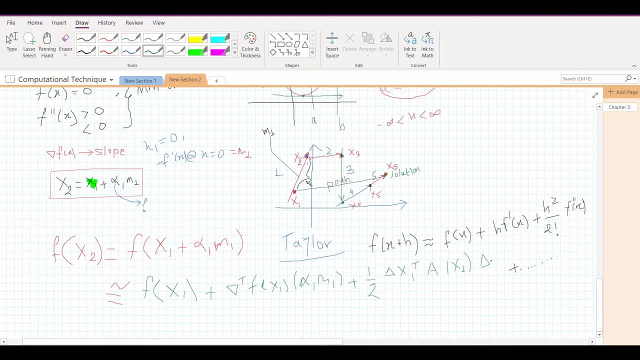 and here, this is how right. derivatives in matrix, this is how right derivatives in matrix, this is how right derivatives in matrix: form, form, form. this means second derivative, this means second derivative, this means second derivative. and we'll have a matrix here, a matrix, and we'll have a matrix here, a matrix. 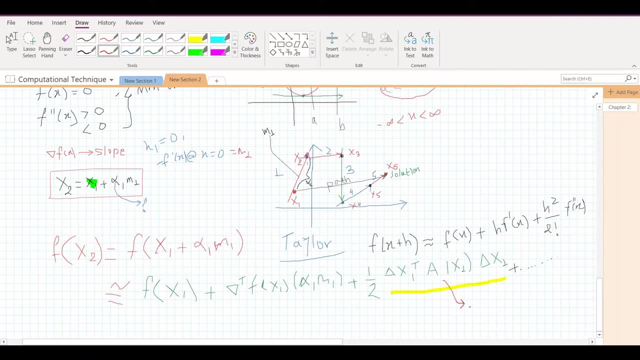 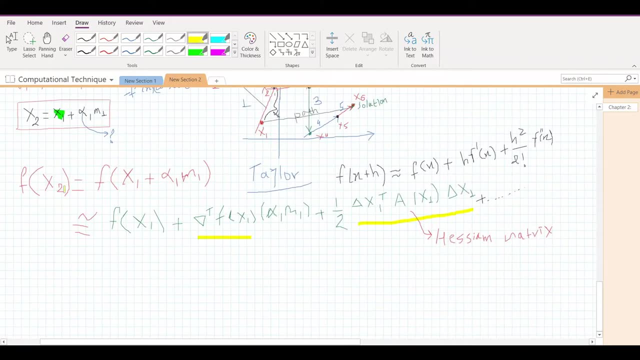 and we'll have a matrix here, a matrix- now this matrix is known as a cn matrix- and then a cn matrix, and then a cn matrix, and then, when we do a derivative of this, when we do a derivative of this, when we do a derivative of this with respect to alpha, 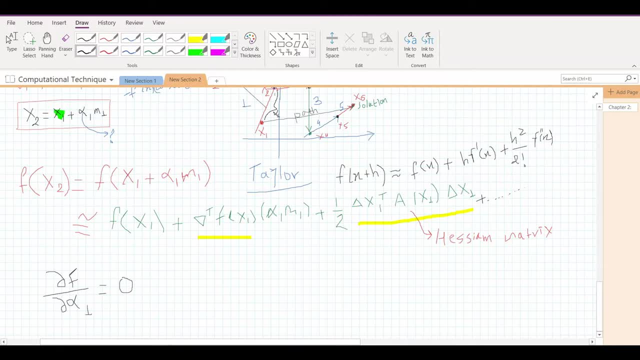 with respect to alpha, with respect to alpha, 1, then equal, that is 0. 1, then equal, that is 0. 1, then equal, that is 0. now, this will give us our step length. now. this will give us our step length. now, this will give us our step length. alpha 1, which we require. 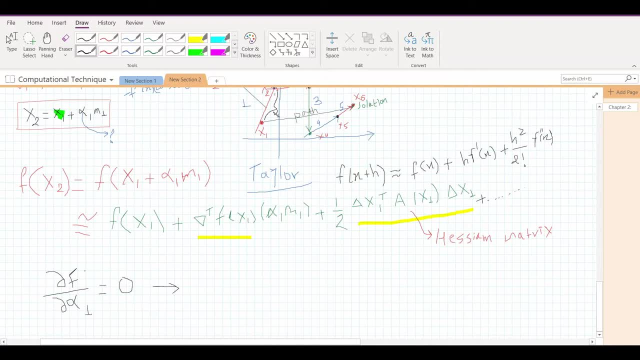 alpha 1 which we require, alpha 1 which we require. the region: we are finding derivative of the region. we are finding derivative of the region, we are finding derivative of function f, function f, function f of x2. with respect to alpha 1, is that: with respect to alpha 1, is that: 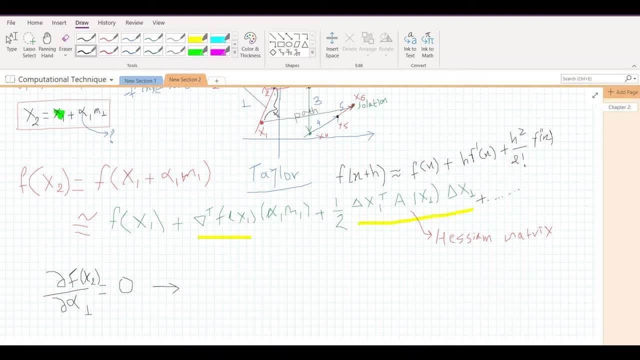 with respect to alpha 1 is that we want to find the minimum length, we. we want to find the minimum length, we. we want to find the minimum length. we have to move, have to move, have to move. this will be, this will be. this will be 0, because there is no alpha 1 term here. 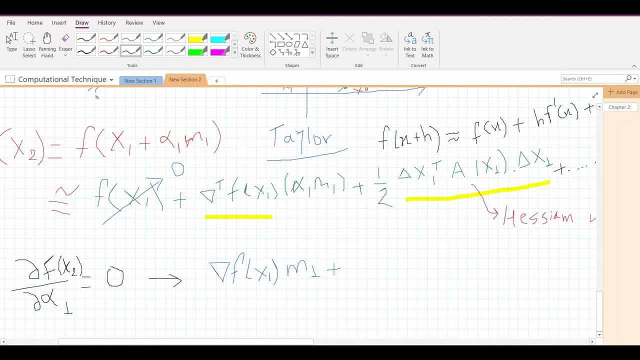 0 because there is no alpha 1 term here. 0 because there is no alpha 1 term here now. this will be now. this will be now. this will be plus here, plus here, plus here, which will be equal to, which will be equal to, which will be equal to 0.. 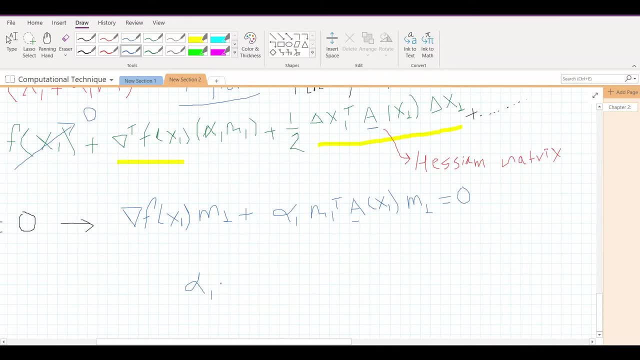 0.. 0.. now, when you solve it, you'll get your. now, when you solve it, you'll get your. now, when you solve it, you'll get your alpha 1, alpha 1, alpha 1, which will be equal to minus. so there you have it. 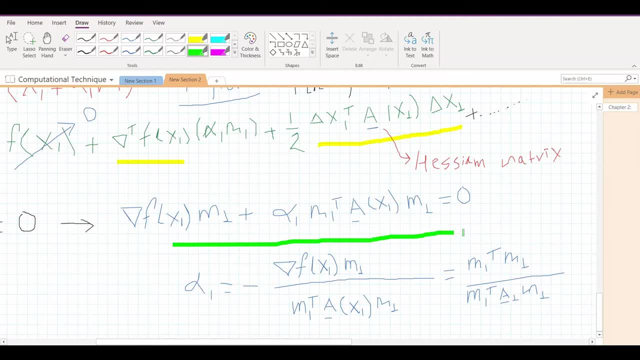 so there you have it. so there you have it. now you have your. now you have your. now you have your alpha as well. this is your step length alpha as well. this is your step length alpha as well. this is your step length there, there, there, therefore, you can have your second. 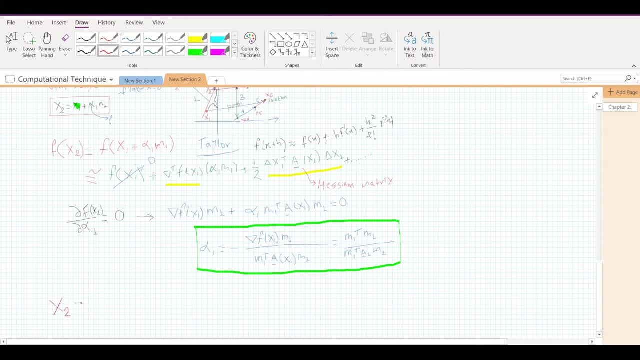 therefore, you can have your second. therefore, you can have your second point now, which is x2, point now, which is x2, point now which is x2, which will be equal to, which will be equal to, which will be equal to x1 plus x1 plus. 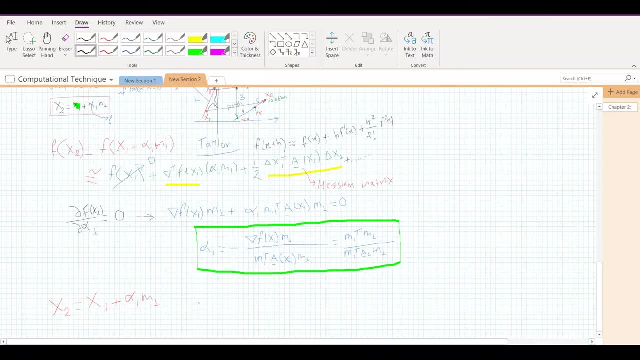 x1 plus alpha 1, alpha 1, alpha 1, m1, m1, m1. in the next step, you will form x3. in the next step, you will form x3. in the next step, you will form x3, which will be equal to. which will be equal to. 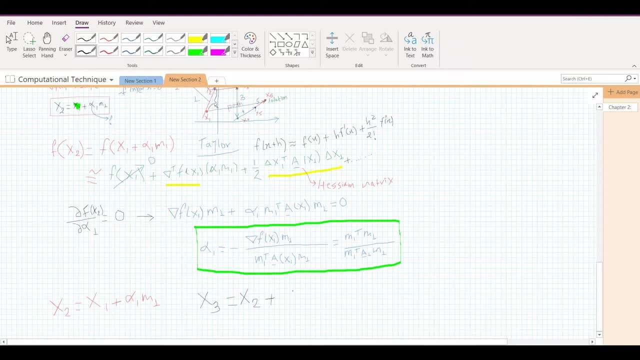 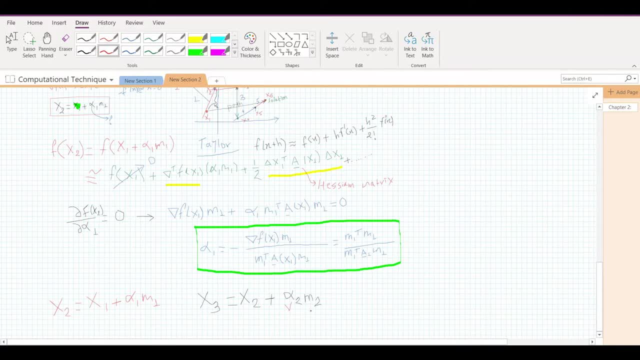 repeat the same procedure here to find. repeat the same procedure here to find your alpha 2, your alpha 2, your alpha 2, m2. and then you have to keep checking if m2, and then you have to keep checking if m2, and then you have to keep checking if the gradient is. 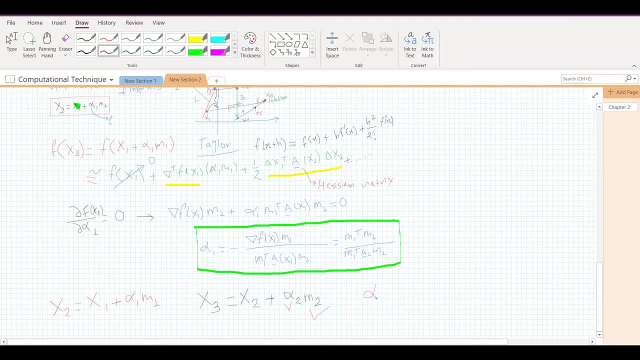 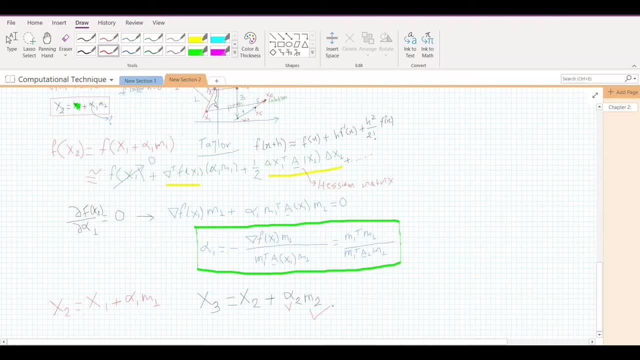 and and you have to keep checking your slope, you have to keep checking your slope, you have to keep checking your slope. if your slope at n, if your slope at n, if your slope at n is not zero, is not zero, is not zero, then you have to move into the next. 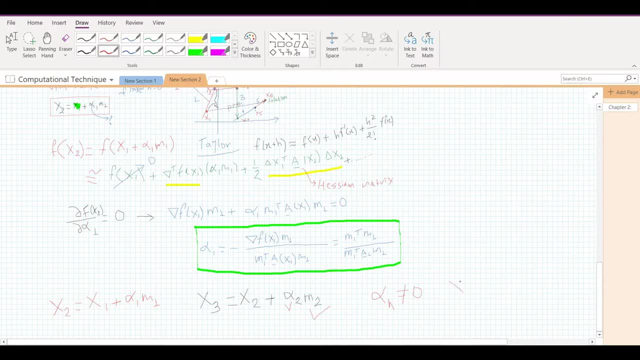 then you have to move into the next, then you have to move into the next step where you will find step where you will find step where you will find x, x, x and plus one otherwise, and plus one otherwise and plus one otherwise, if you're, if you're. 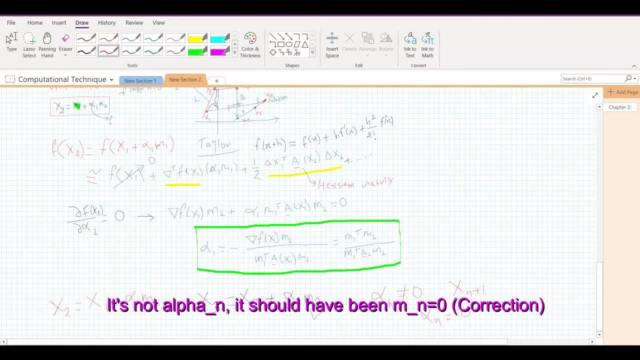 if you're a cost to zero, then you'll have your a cost to zero, then you'll have your a cost to zero, then you'll have your solution: as x as x, as x and minus one, and minus one and minus one. we'll see this when you do an. 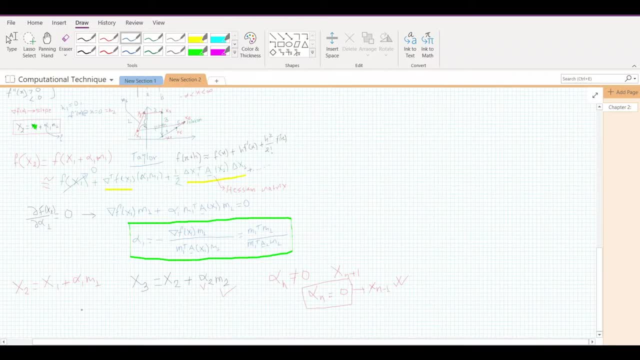 we'll see this when you do an. we'll see this when you do an example. this kind of procedure is known as example. this kind of procedure is known as example. this kind of procedure is known as steepest gradient method, the major. steepest gradient method, the major. 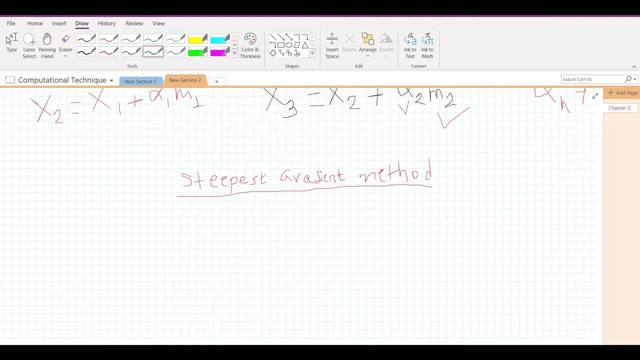 steepest gradient method. the major problem with steepest gradient method is problem with steepest gradient method is problem with steepest gradient method is that it generally takes a lot of that. it generally takes a lot of that. it generally takes a lot of iterations to solve. 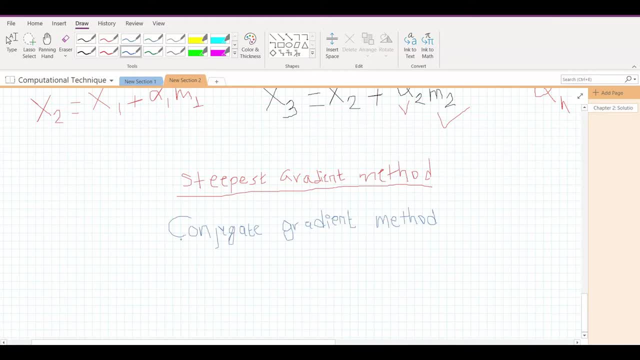 iterations to solve. iterations to solve a problem, a problem, a problem as such. conjugate gradient method as such, conjugate gradient method as such. conjugate gradient method came into picture here the conjugate came into picture. here the conjugate came into picture here the conjugate gradient method. 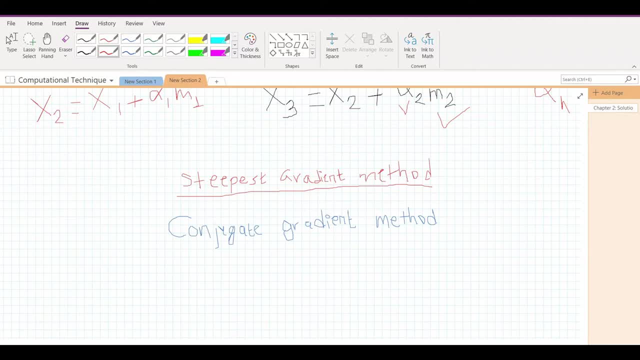 gradient method. gradient method helps to reduce the number of, helps to reduce the number of, helps to reduce the number of iterations to solve the problem. iterations to solve the problem, iterations to solve the problem. let's take the same example that we. let's take the same example that we. 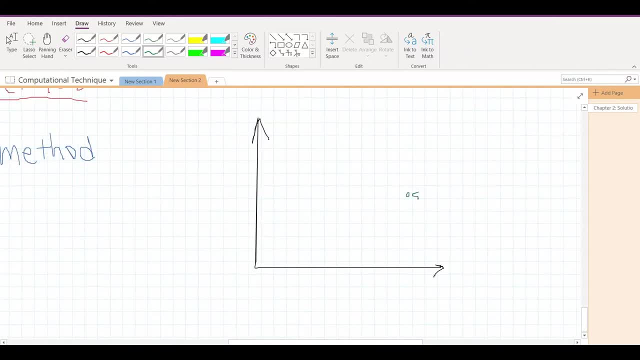 let's take the same example that we took here, if this point was our required, took here if this point was our required, took here, if this point was our required: solution, solution, solution. what to do here is if you take this one, what to do here is if you take this one. 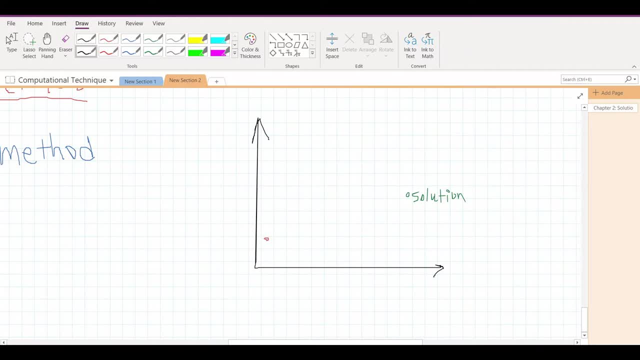 what to do here is, if you take this one as initial guess, as initial guess, as initial guess, then we'll get a slope like this, then we'll get a slope like this, then we'll get a slope like this, and then, and then, and then another slope. 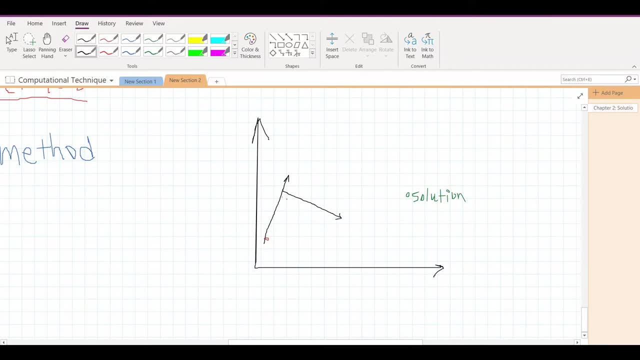 another slope, another slope will be, will be, will be perpendicular, perpendicular, perpendicular to the first slope. and then we'll reach a point here, and then we'll reach a point here, and then we'll reach a point here. from here, we'll reach a point here. from here, we'll reach a point here. 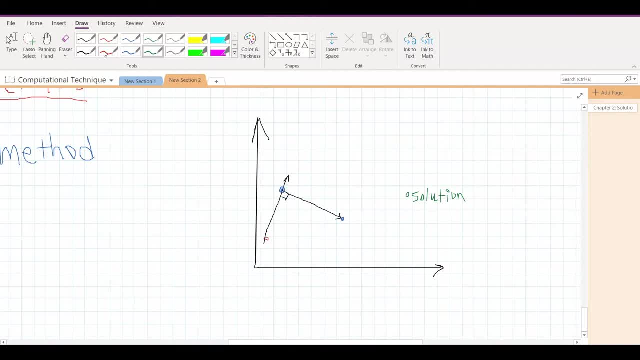 from here we'll reach a point here, and then from here we will, and then from here we will, and then from here we will reach another point, reach another point, reach another point, and then, and then, and then, from here, from here, from here, like this, like this: 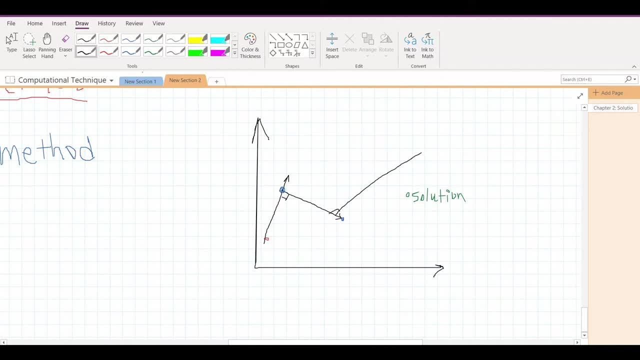 like this, which will also be 90 degree, which will also be 90 degree, which will also be 90 degree to a point, to a point, to a point here, here, here, and then, and then, and then, from, from, from here, here, here to here, we define a specific path to our 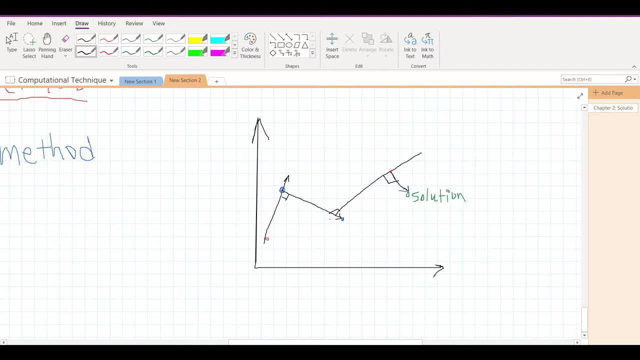 to. here we define a specific path to our to. here we define a specific path to our iteration, iteration, iteration. this drastically reduces the number of this drastically reduces the number of this drastically reduces the number of steps. these slopes are not steps. these slopes are not steps. these slopes are not directly perpendicular or conjugate as 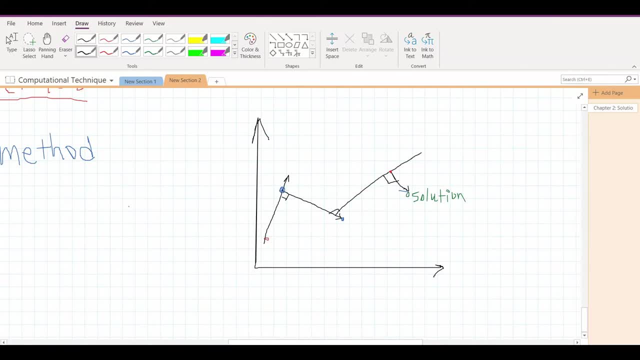 directly perpendicular or conjugate, as directly perpendicular or conjugate, as you see here, but they are conjugate. you see here, but they are conjugate, you see here, but they are conjugate. respect to a certain respect, to a certain respect to a certain matrix, matrix, matrix which is known as the asian matrix a. 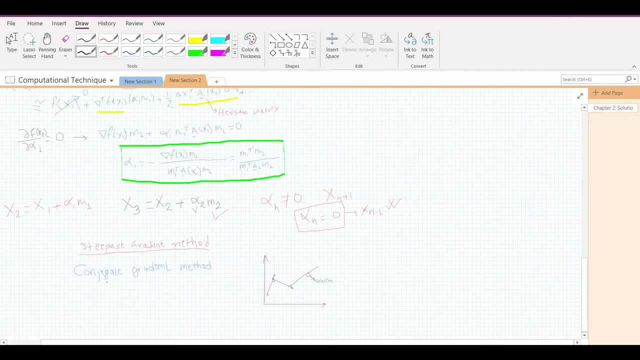 which is known as the asian matrix a, which is known as the asian matrix a, which is a here, which is a here, which is a here. so so, so, what will happen here is that what will happen here is that what will happen here is that we have to find. 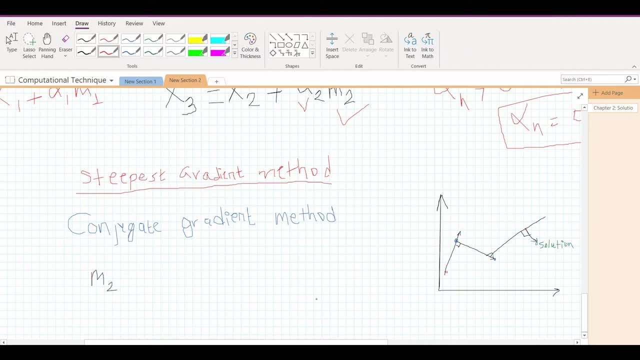 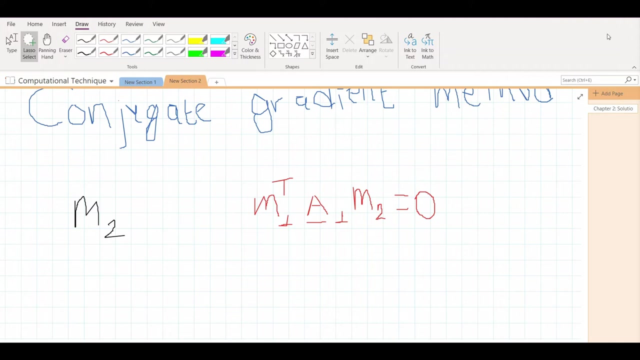 we have to find. we have to find m2, which is our next slope. this one, m1 and m2 are conjugate with respect to asian matrix, now in the asian matrix, now in the asian matrix, now in the conjugate gradient method. conjugate gradient method. 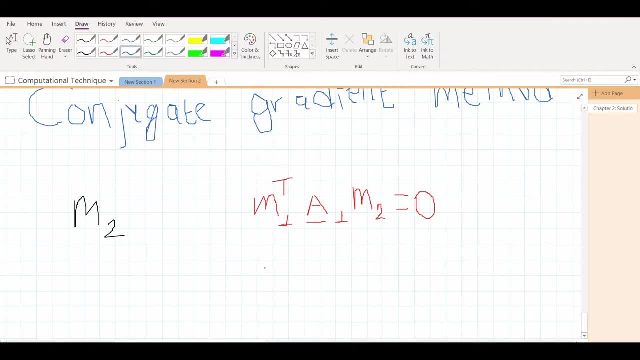 conjugate gradient method. what we assume is what we assume is. what we assume is or m2 or m2, or m2 is linearly varying with respect to m1. linearly varying with respect to m1. linearly varying with respect to m1, as. 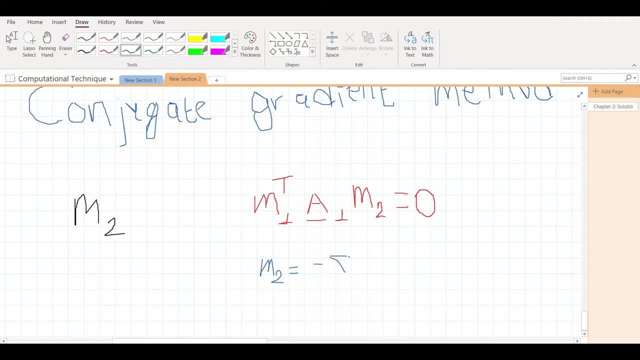 minus gradient, as minus gradient, as minus gradient of of of f2, f2, f2 plus beta, 2 m m m, 1 m1 m1. now we can substitute this here, and then now we can substitute this here and then now we can substitute this here and then solve it. 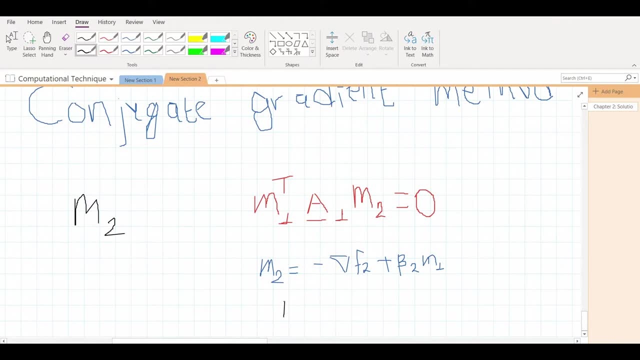 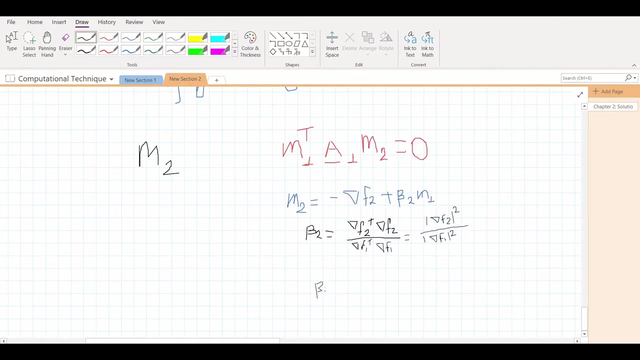 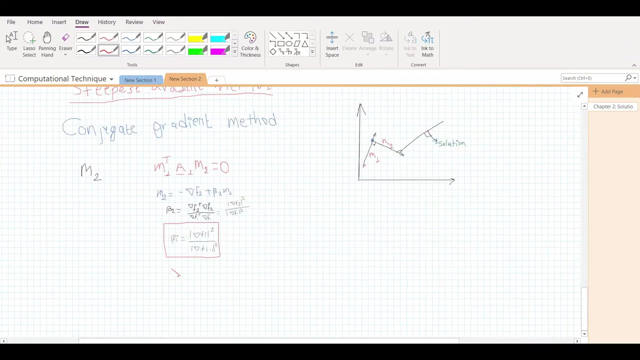 solve it. solve it. the result will be something like this: we'll. the result will be something like this: we'll. the result will be something like this: we'll get, get, get. beta 2 will be equals to. similarly, your beta i will be equal to. therefore, you can obtain your m2, so your. 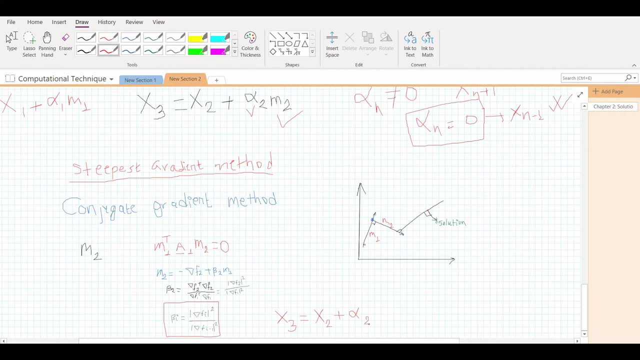 therefore, you can obtain your m2, so your. therefore you can obtain your m2, so your x3, x3, x3 here will be equal to m2. now your m2 will be this one here, and then you can repeat your procedure, and then you can repeat your procedure. 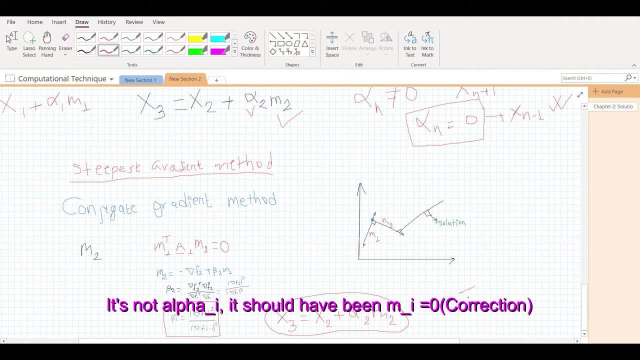 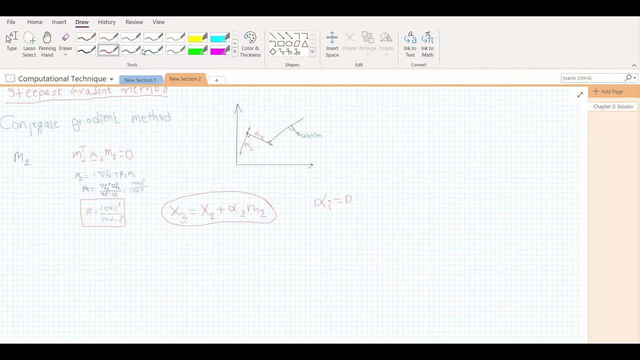 and then you can repeat your procedure again and again, and again, again and again and again, until you have, again and again, and again, until you have, again and again and again, until you have alpha i, alpha i, alpha i, equals to equals to equals to zero, zero, zero now in conjugate gradient method: 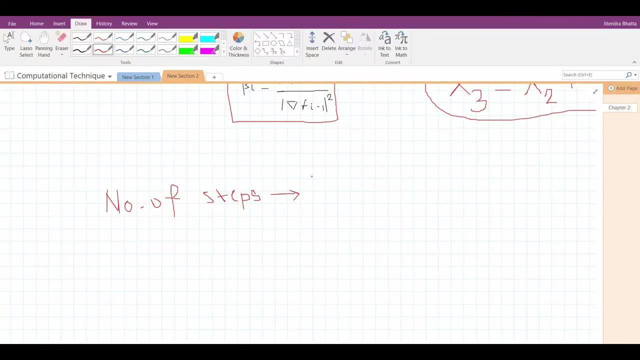 now in conjugate gradient method. now in conjugate gradient method, the number of steps that are required, or the number of steps that are required, or the number of steps that are required or the number of iterations to solve a. the number of iterations to solve a. the number of iterations to solve a problem. 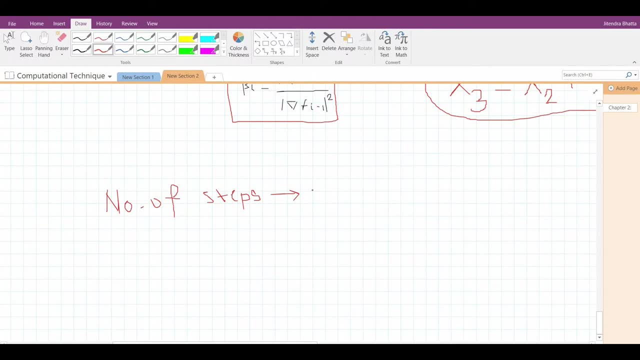 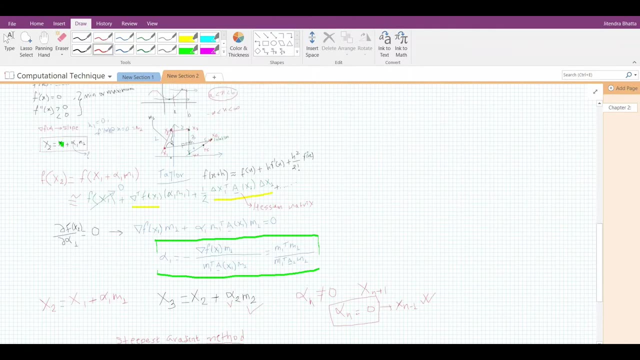 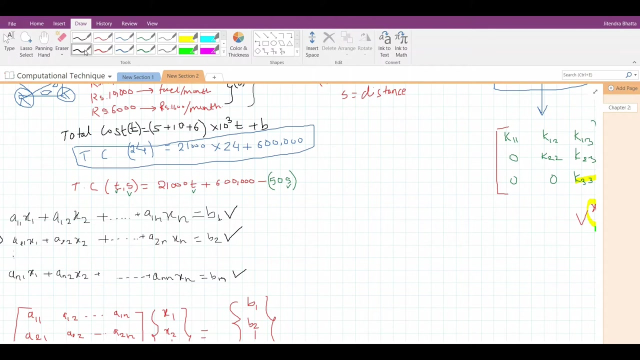 problem problem depend upon the number of variables, which depend upon the number of variables, which depend upon the number of variables which are known as decision variables, are known as decision variables. are known as decision variables, for example, for a problem like this one, and we have like this one, and we have 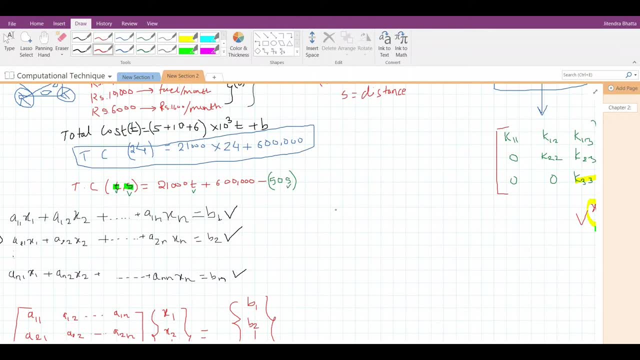 like this one and we have two variables, t and s, two variables t and s, two variables t and s, then the number of steps that the, then the number of steps that the, then the number of steps that the conjugate gradient method, conjugate gradient method, conjugate gradient method will take will be two. 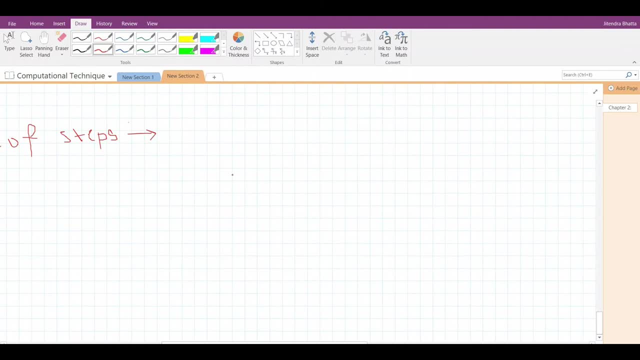 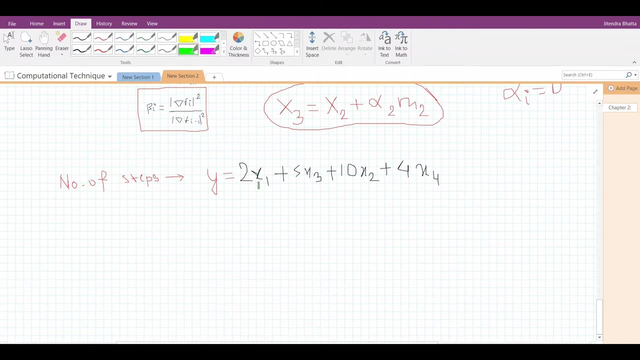 will take will be two. will take, will be two. similarly, similarly, similarly. when you have an equation like, when you have an equation like, when you have an equation like, like this y equals to, then you can see here that there are x1, then you can see here that there are x1. 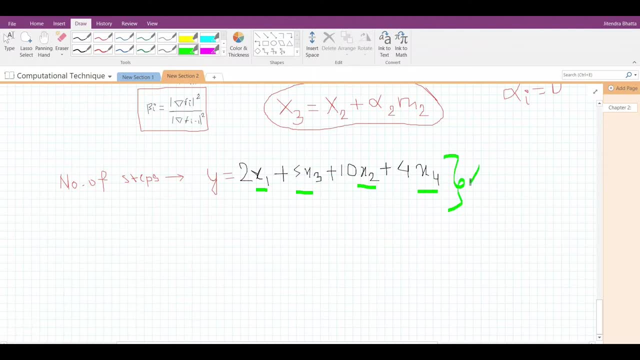 then you can see here that there are x1, x2, x3 and x4. so there are four: x2, x3 and x4. so there are four: x2, x3 and x4. so there are four variables. therefore, the maximum number of variables, therefore, the maximum number of 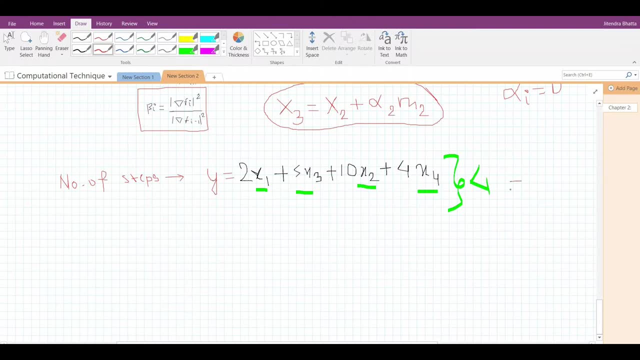 variables. therefore, the maximum number of steps, steps, steps to solve this problem will be equal to: to solve this problem will be equal to: to solve this problem will be equal to four, four, four. now. this is one of the advantages of now. this is one of the advantages of. 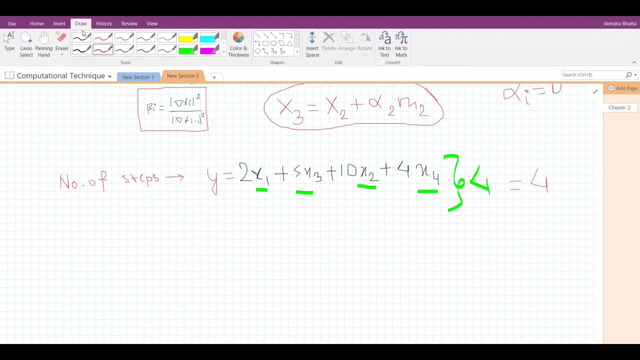 now, this is one of the advantages of conjugate gradient, conjugate gradient, conjugate gradient method. this method is also known as method. this method is also known as method. this method is also known as fletcher-reves method. now let's look at fletcher-reves method. now let's look at 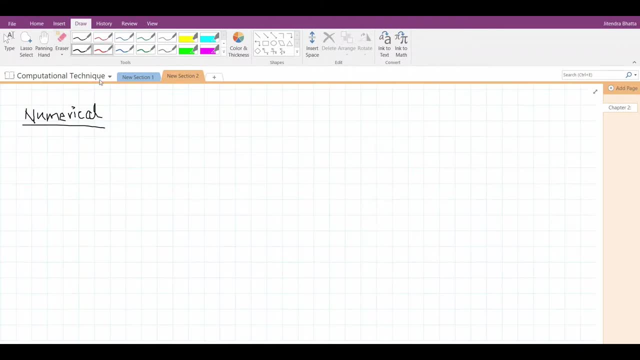 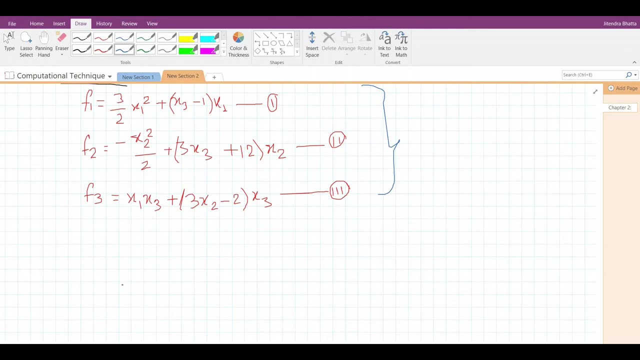 fletcher-reves method. now let's look at an example, an example. an example example will make everything clear. let's say you are given three equations. let's say you are given three equations. let's say you are given three equations to solve, to solve, to solve. what i define first is the gradient of. 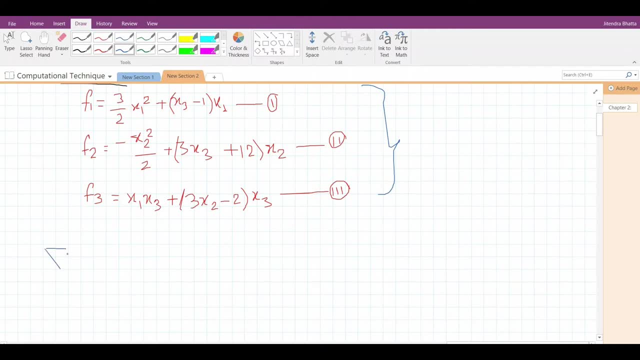 what i define first is the gradient of. what i define first is the gradient of these functions. so the gradient these functions, so the gradient of these functions, so the gradient of these functions, so the gradient these functions, so the gradient of these functions. so the gradient f will be equal to. 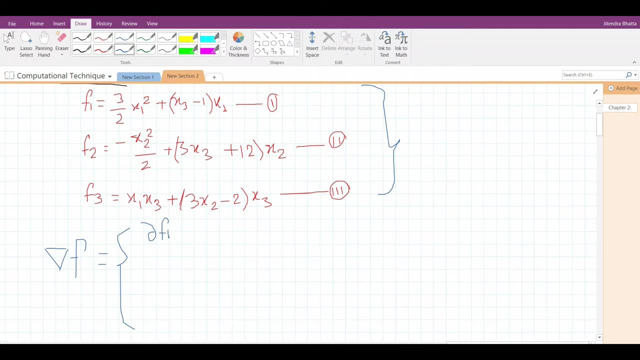 derivative of function, one with derivative of function, one with derivative of function, one with respect to x1, and then here derivative of function x1, and then here derivative of function x1, and then here derivative of function 2. 2, 2 respect to x2. 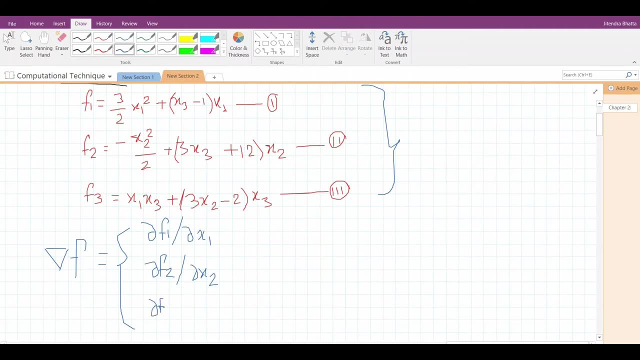 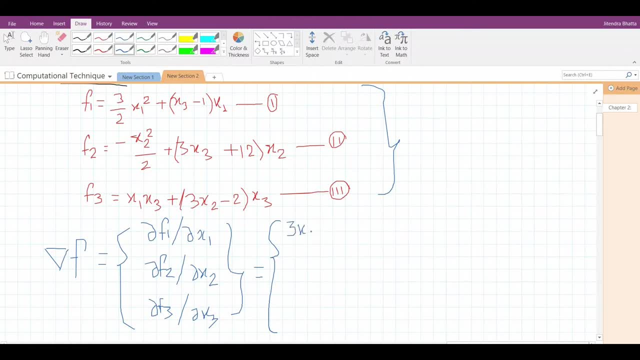 if we do a derivative here, 3, x1 plus x3, x3, x3, x3 minus 1 minus 1, x3 minus 1, this one, this one, this one will be equal to minus x2, will be equal to minus x2, will be equal to minus x2 plus 3. 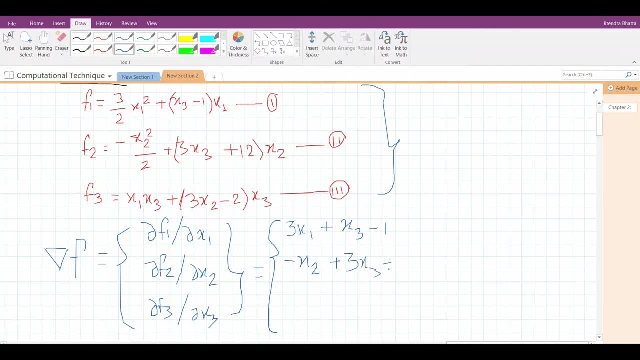 plus 3 plus 3, x3, x3, x3 plus 12 plus 12 plus 12, and the third one here with respect to x3, and the third one here with respect to x3, and the third one here with respect to x3, you get: 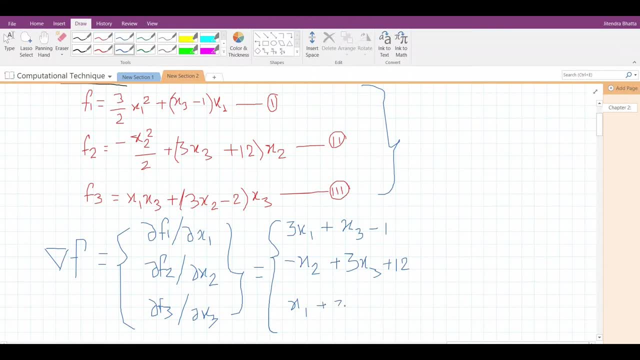 you get? you get x1 plus x1 plus x1 plus 3x, 3x, 3x, 2, 2, 2, 2 ands 1, 2, 2. now this is your gradient 2. now, this is your gradient 2. now this is your gradient. 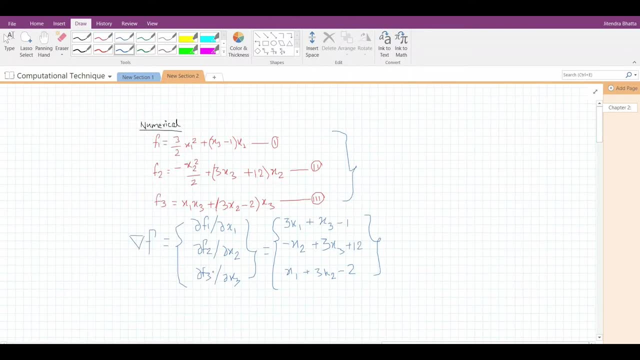 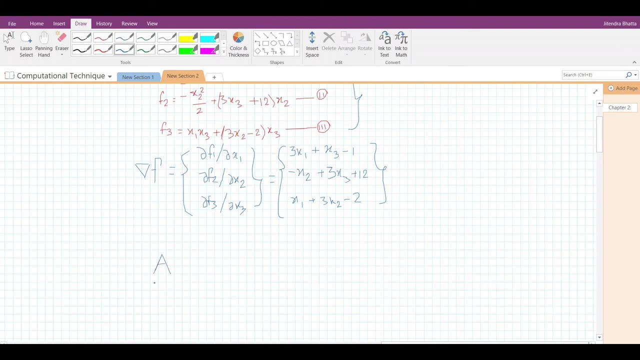 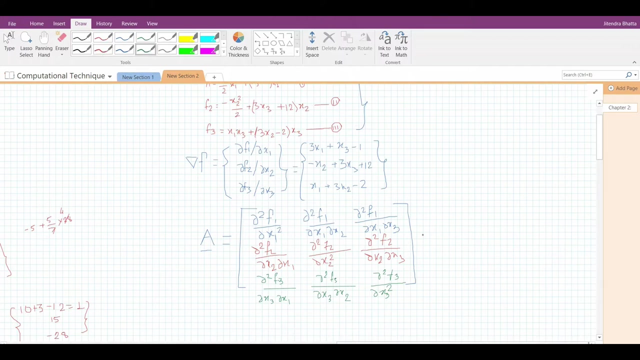 and then here to find your hcn matrix, which is given by this equation. now, this will be your a matrix. now, this will be your a matrix. let's find our a matrix, which will be equal to. we have to find derivative of this one two times with respect to x1, so this will give us three. 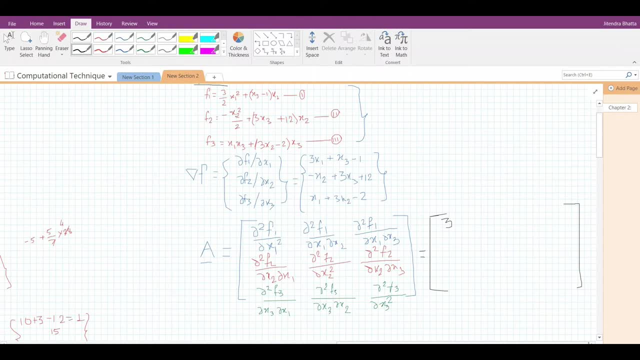 here we do it first with x2, which is zero, and then this one with respect to x3 will give us x1, and the respect to x1 will give us one again. this one with respect to x1 first will give us zero, and for this one 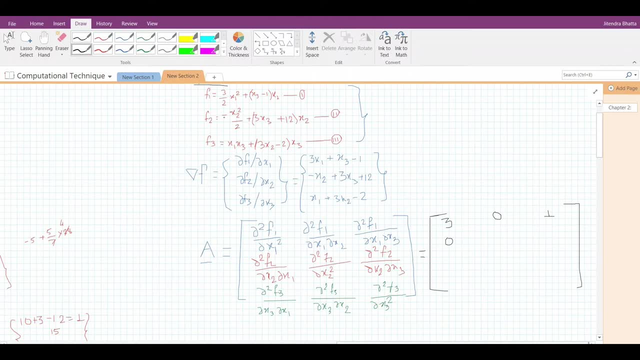 with respect to x2, 2 times will give us minus 1, and then for this one x 3, because x2 will give us 3x2, and then this will be equal to 3. here, first we want to find derivative with respect to x1, which will be x3, and then with: 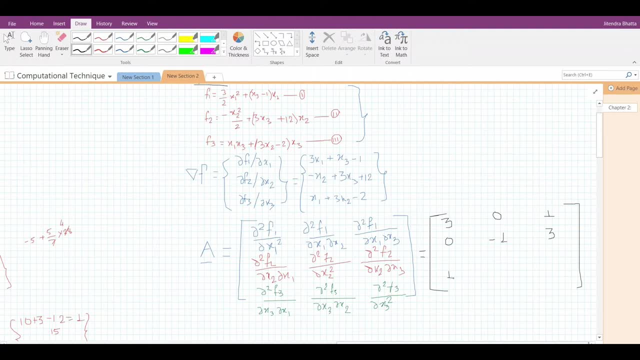 x3, it will be zero, and then we will look for derivative of x1, which is 1.. present probably here with respect to x2, which is equal to one, and then with the x2 it'll be x3, and then 1. 1 here, first with X 2. this will give us 3, X 3, and then, with respect to X, 3 will. 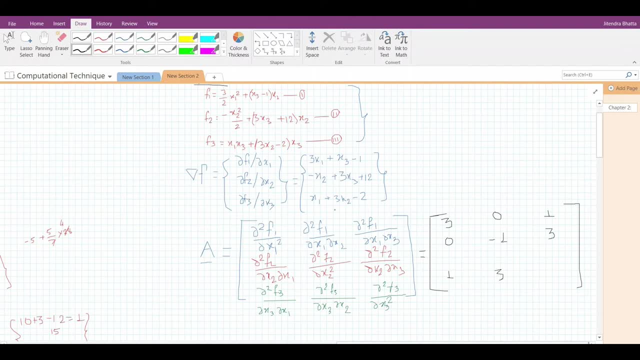 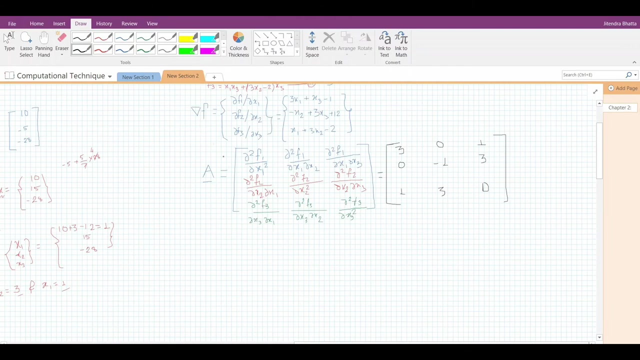 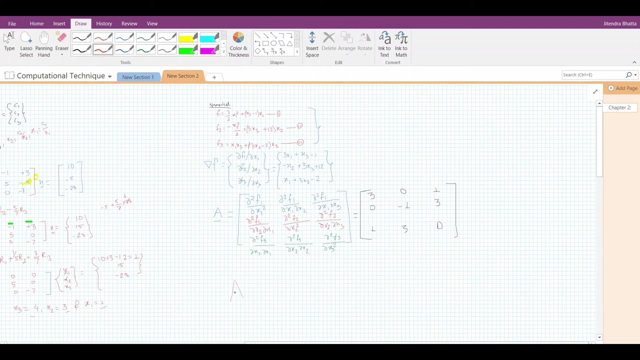 give us 3, and here this one with respect to X, 3 2 times will give us 0. this is your Haitian matrix. this is your gradient vector in your examination. similar type of problem will be given to you in form of AX equals to B, so you'll. 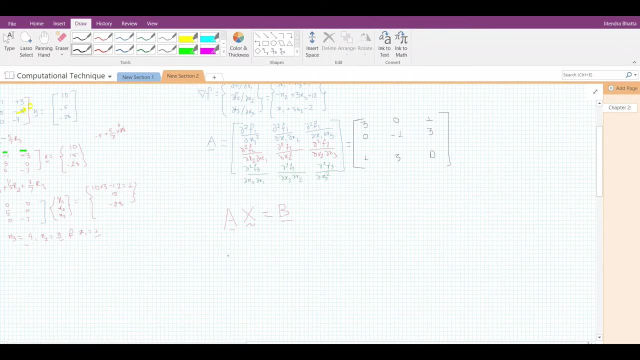 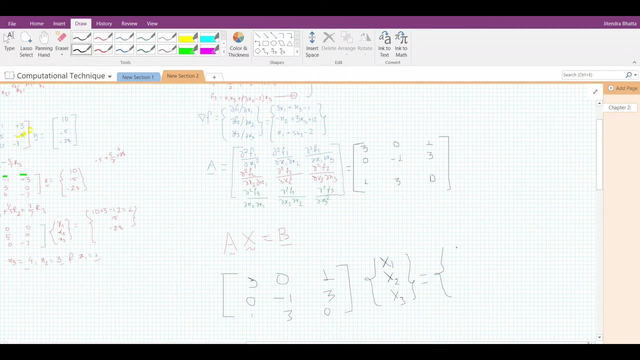 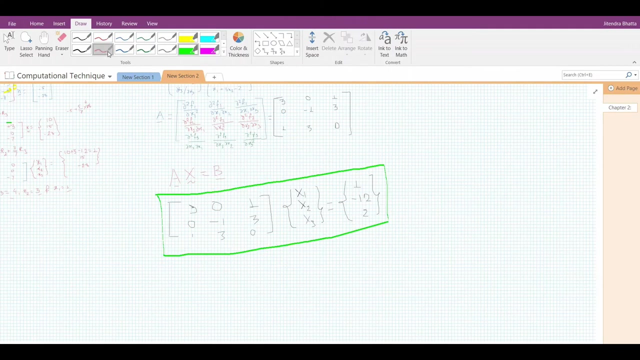 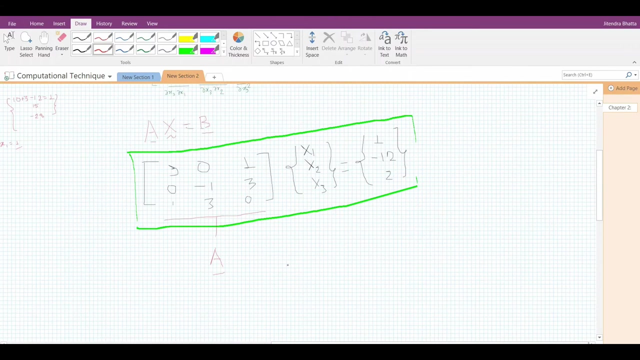 be given to solve this problem like this here. this one will be: when you take this one to the right side, it will be 1 minus 12 and 2 you. so in your examination, you will directly be given this equation to solve. we take this one as our Haitian matrix. this is our variables, which you have to solve. 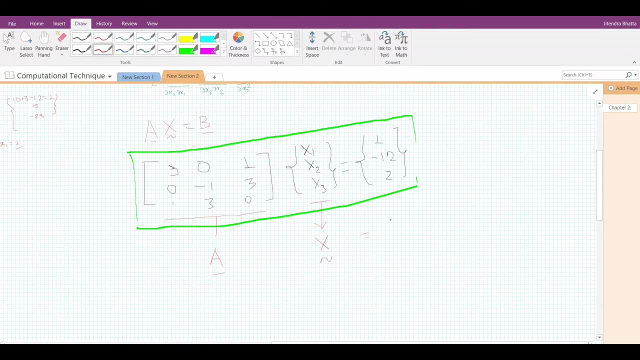 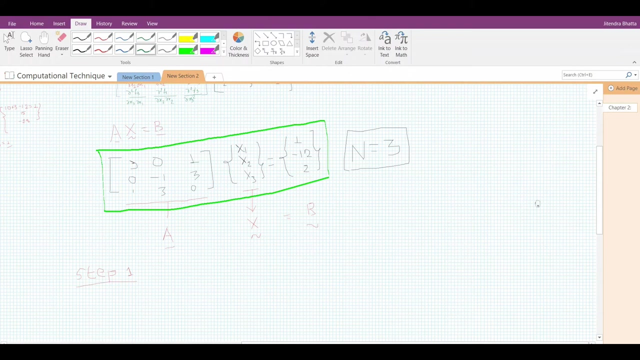 and this one can be taken as B vector. so we start from here, step one. as you can see here that there are three variables, so the maximum number of iterations to solve this problem will be equal to 3.. here the exact solution lies somewhere here and therefore we have to assume a point somewhere here. let's say: 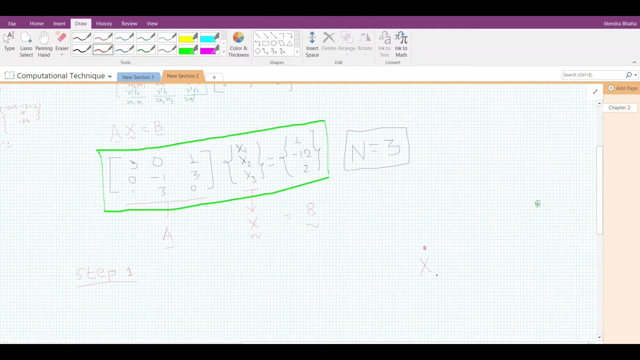 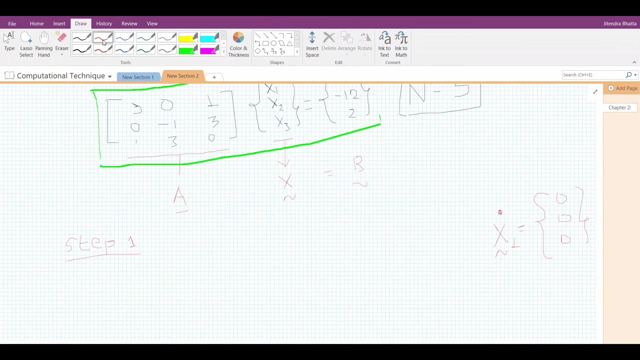 this is our first point. we have assumed X 1 vector as 0 and 5 and n options. whether we are using those terms or not goes down this time 0 0, 0. then what we have to find here is we have to find our gradient at 0 0, 0 to. 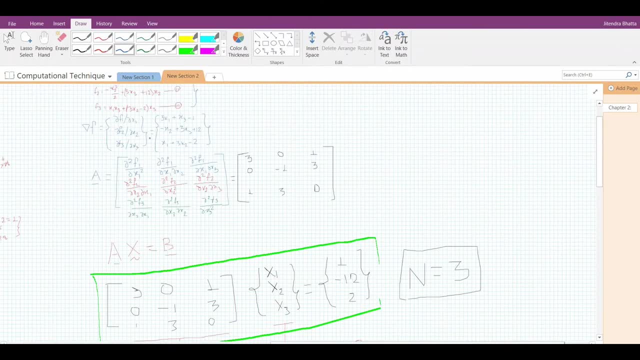 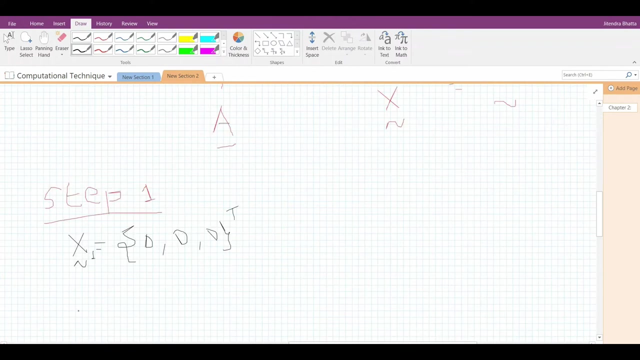 find the gradient 0 0 0. see the equation we have derived here. we'll use this equation. so when you substitute 0 0 0 here, what do you get? you get minus 1 plus 12 and minus 2 here. right, your M 1. 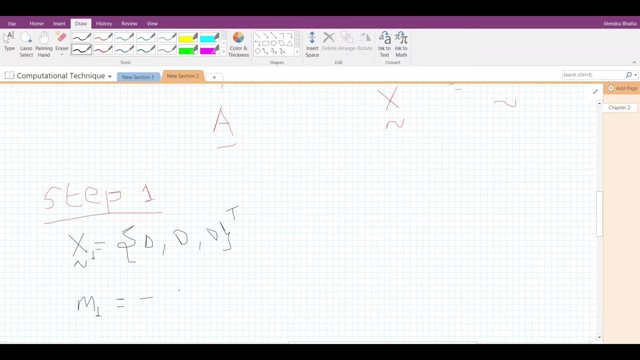 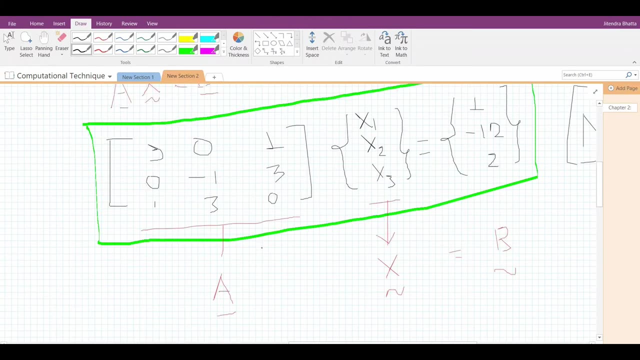 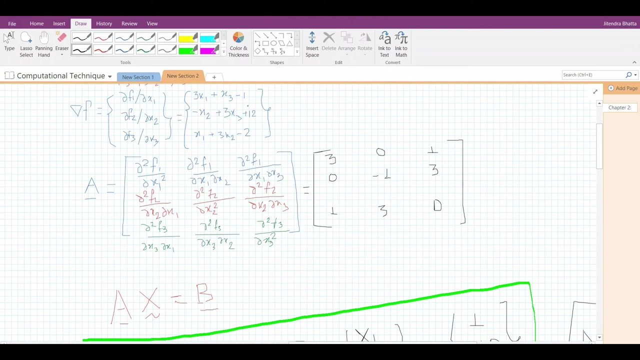 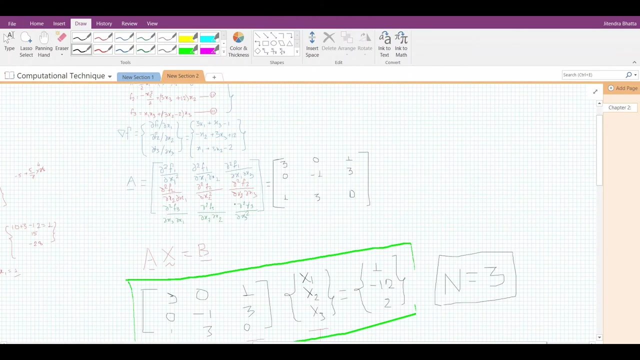 will be equal to negative of gradient of F 1. we have to substitute 0 0, 0 in here to obtain our gradients. now this vector, as you can see here, equals to the negative of B vector in your equation, so this one will be equal. 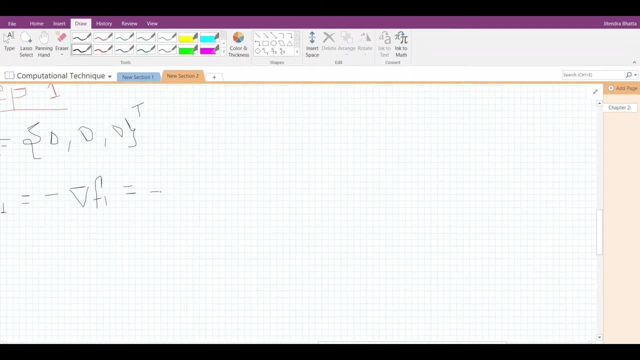 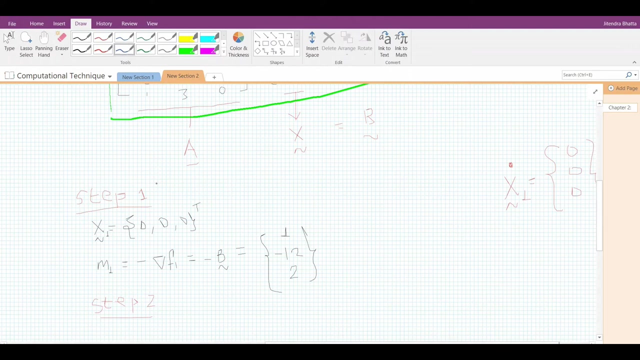 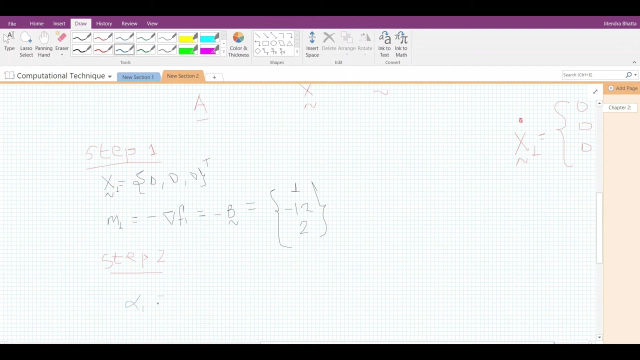 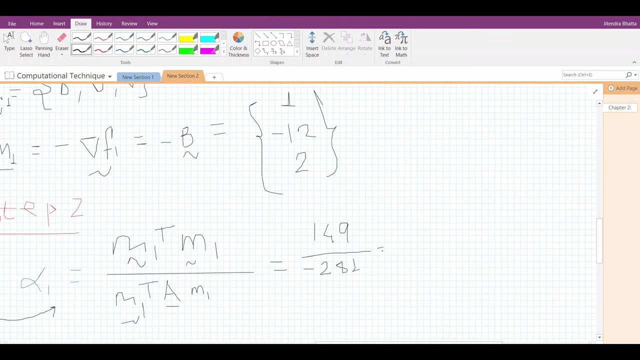 to negative of B 1 B vector, so this one will be equal to. now this is our m1. step 2 is to find our step. our step is alpha 1, which will be equal to: so this is our alpha 1. so we write here: and this is equal to minus 0.5302. and the third step: 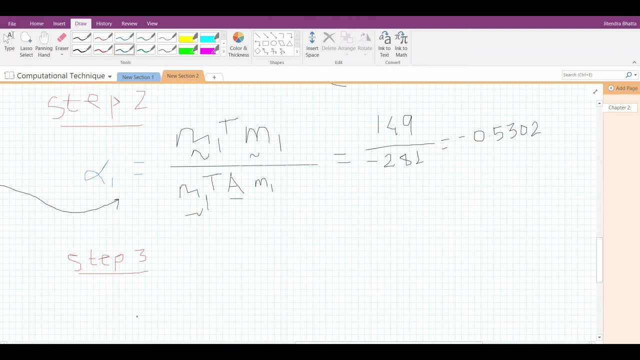 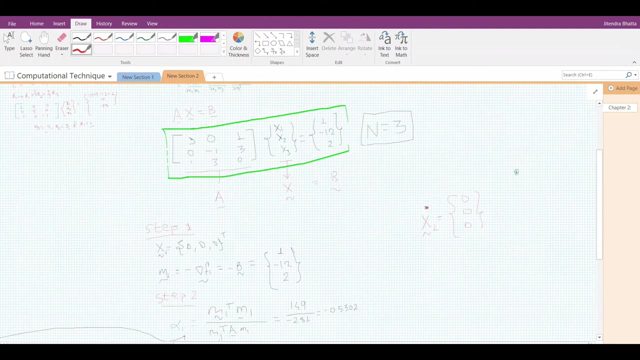 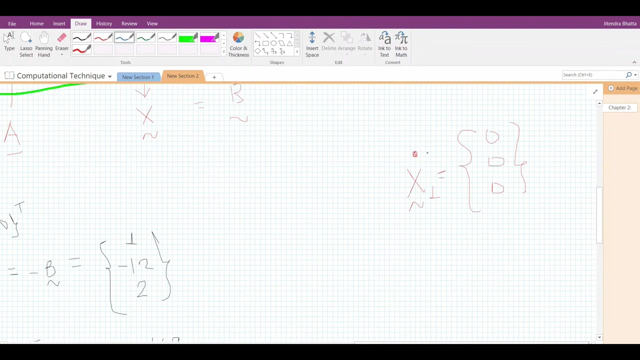 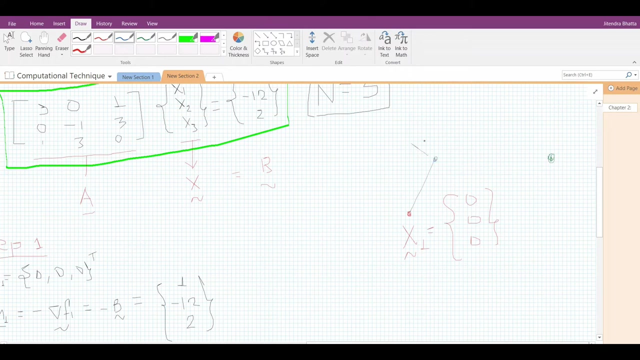 is to find x2 which will be equal to. this means that we started here and we have reached another point somewhere here: x2 using alpha 1, m1. now we have to find another point which will be equal to x3, where we have to use alpha 2, m2 and beta 2. let's find this point or m2, for. 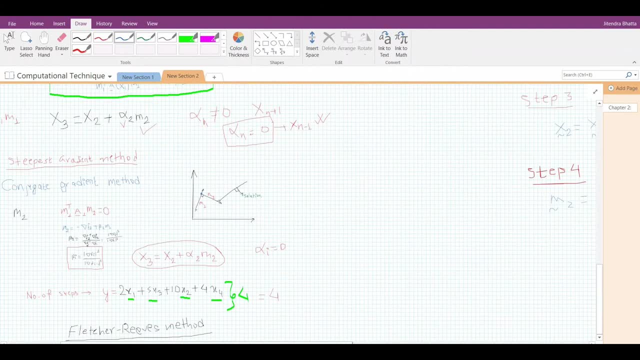 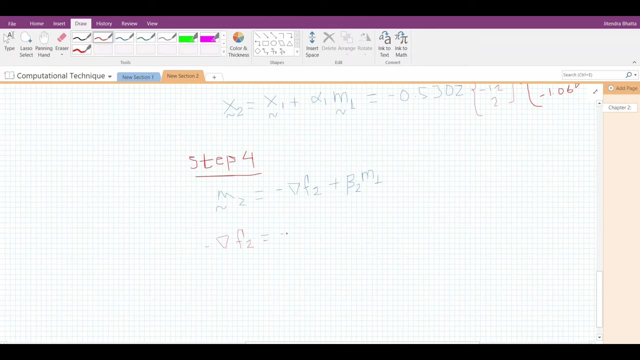 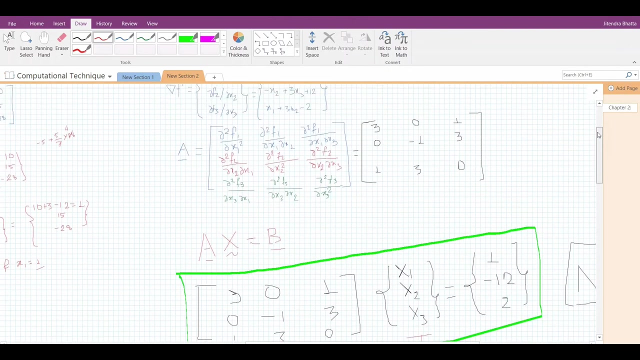 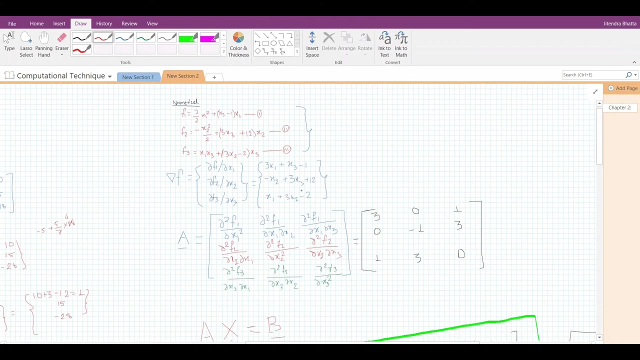 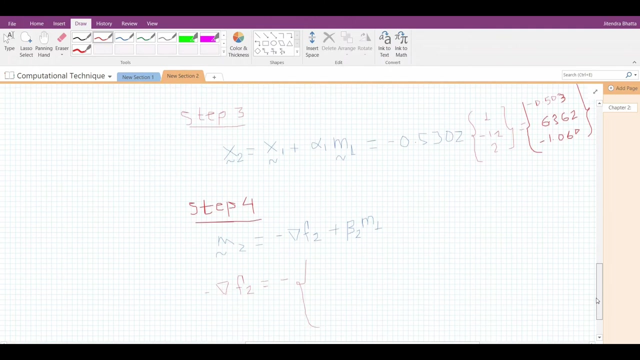 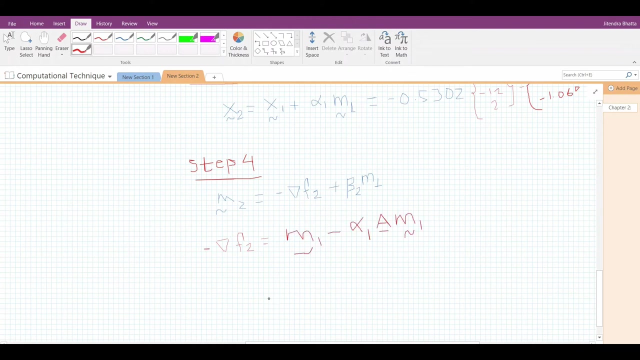 this case equals to this one here will be equal to negative of now. at that point, at x1, y1, y2, were to put these values here and obtain our values. if you are not given these equations here, the equation to find your gradient will be equal to. 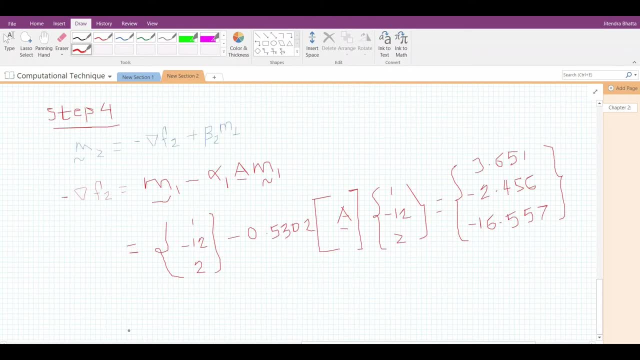 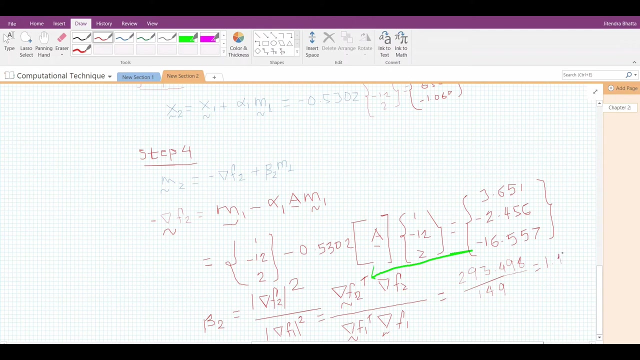 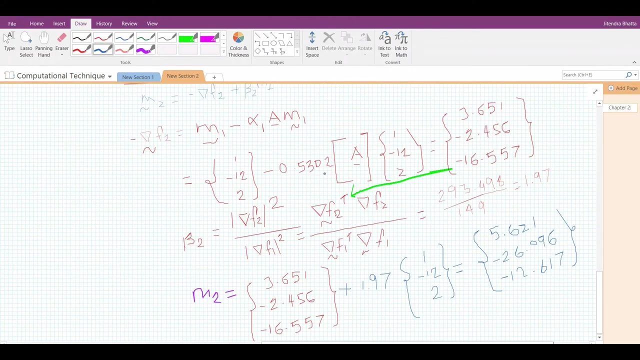 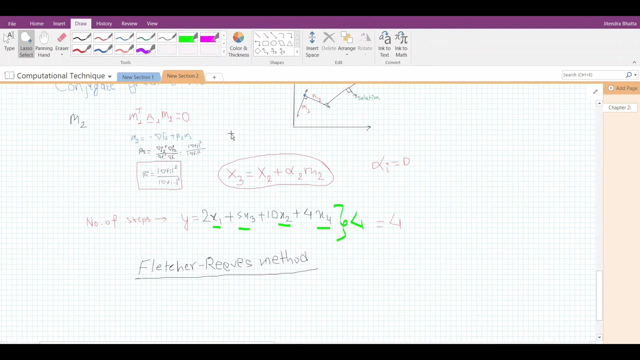 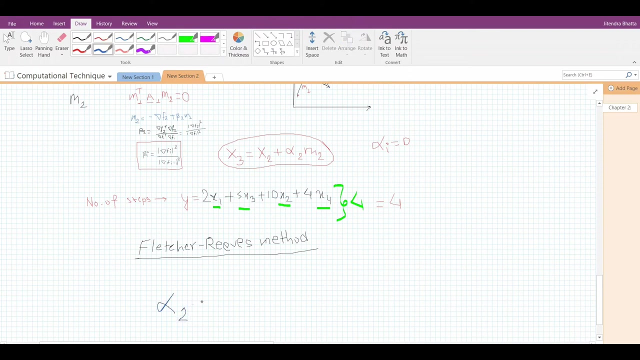 one pole machine. then you have to find your pete two, which will be equal to one point vs one boys nine, seven. therefore your m2 will be equal to again, alpha 2 would be six. I forgot to mention here about alpha 2. to find alpha 2, this will be equal to. 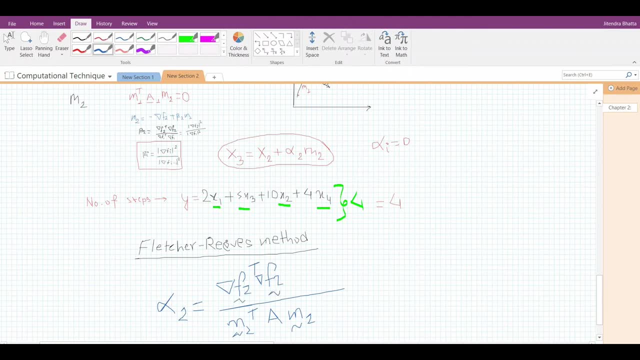 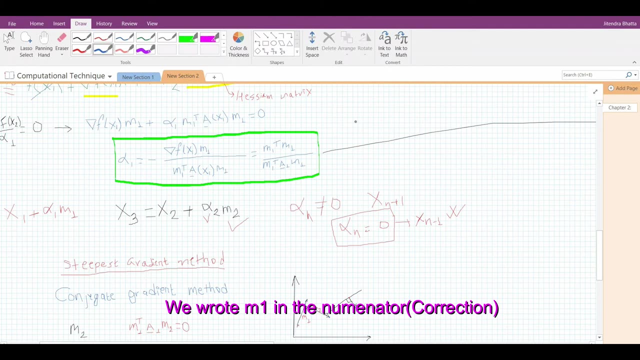 these are all vectors. so in the first case what we did here was we wrote m2, because we assume the initial point to be 0 0, 0. therefore this derivative here turns out to be equal to m1. but here this doesn't happen because we're 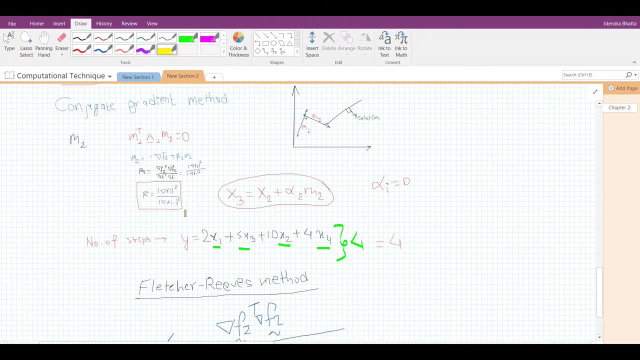 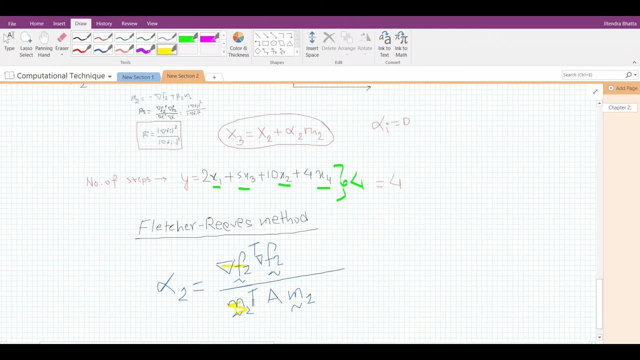 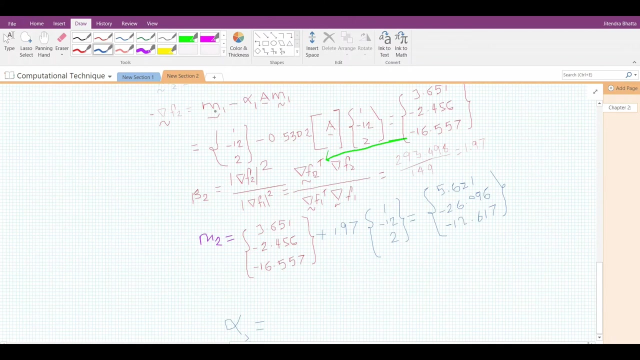 assuming our initial point to be x1 rather than 0 0 0, therefore this- and this will vary for this case- alpha 2 will be equal to this matrix transpose of itself, which will be equal to same as this one here, and then, divided by now, this will be: 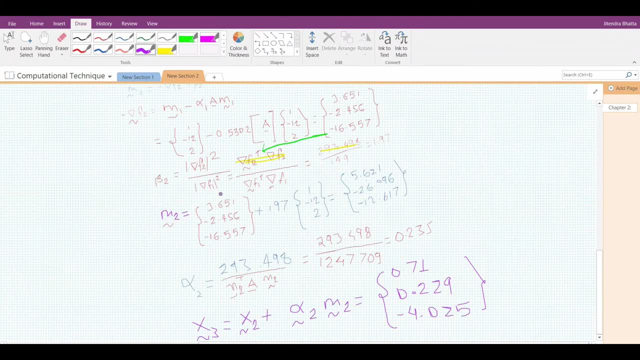 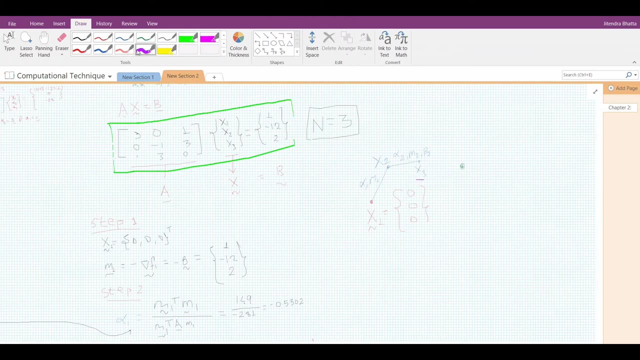 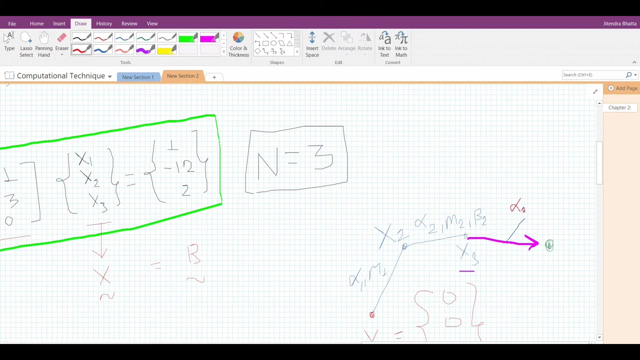 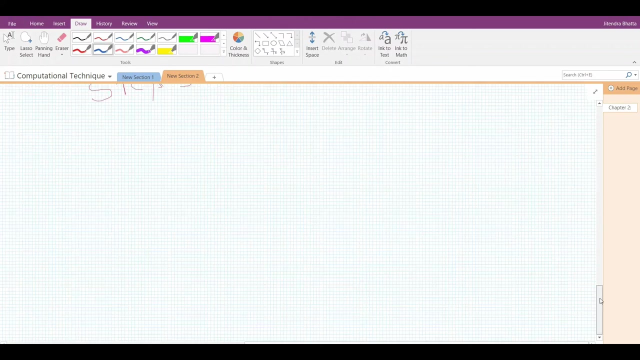 our alpha 2, our x3. now, this is our second iteration, where we have reached here. now, this should be one more step left that will lead us to this point here for this. similarly, we have to find out what is our alpha 3, m3 and beta 3 by